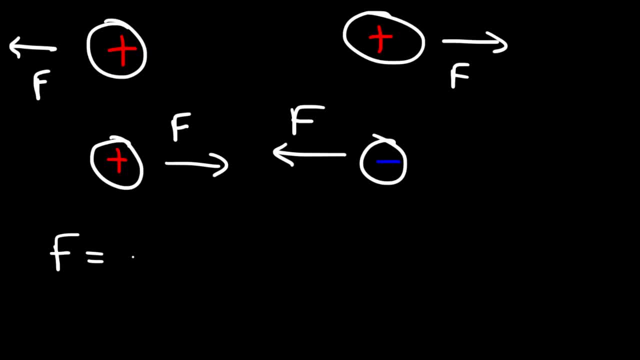 here it is. So the electric static force between two charges is the force of attraction. It's equal to K times Q1 times Q2 divided by R squared Now, K is a constant, It's equal to 9 times 10 to the 9.. And the units are Newtons times square, meters per Coulomb square. 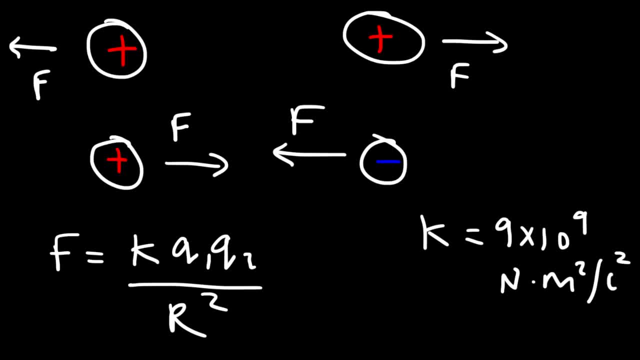 So that's just a fixed value. Now, Q represents the electric charge And Q is measured in Coulomb's Law. R is the distance between the charges. And now let's think about what this equation tells us. If we were to increase the magnitude of, let's say, let's call this Q1 and Q2.. 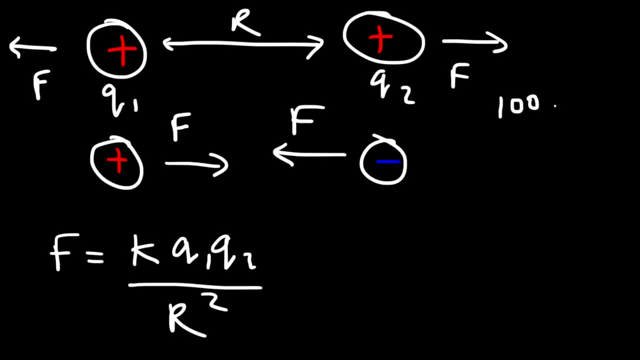 So let's say Q2 increased from 100 microCoulombs to 200 microCoulombs, What do you think the magnitude of the force will be Between the two charges If you increase the magnitude of the charge, the electrostatic? 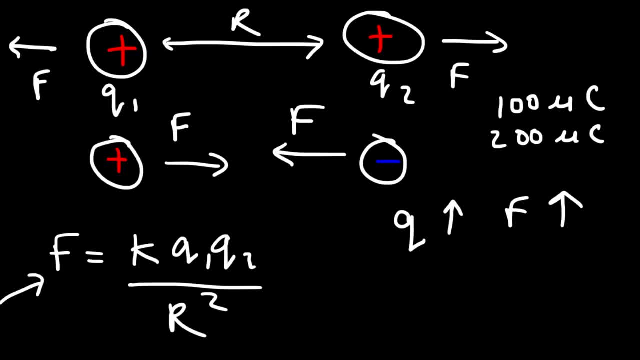 force between the charges will increase. In fact, if you double Q2, then F will double in value. If you double Q1, F will double in value as well. If you double both Q1 and Q2, F will increase by a factor of 4, because 2 times 2 is 4.. 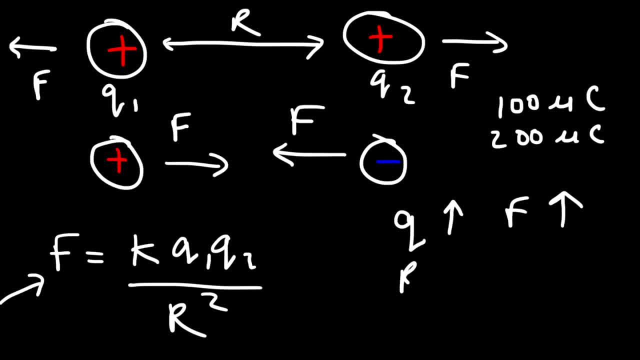 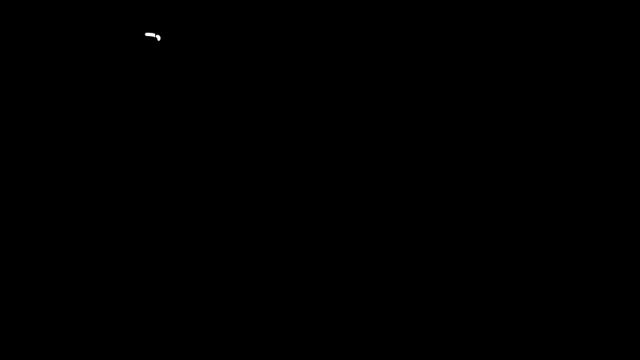 Now what happens if you increase the distance between the two charges? So let's say: here's charge 1 and here is charge 2.. Now let's say the force that's acting on each charge is 100 Newtons when the distance between them is 1 meter. 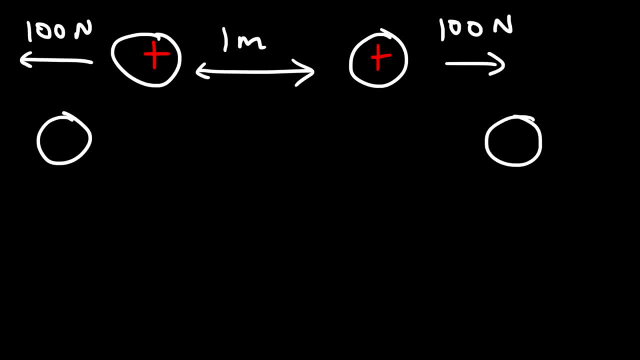 What's going to happen if we double the distance between the two charges, while the magnitude of the charge is still the same? So now the separation distance is 2 meters, Will the electrostatic force acting on the charges increase or decrease? Well, because the charges are further away. 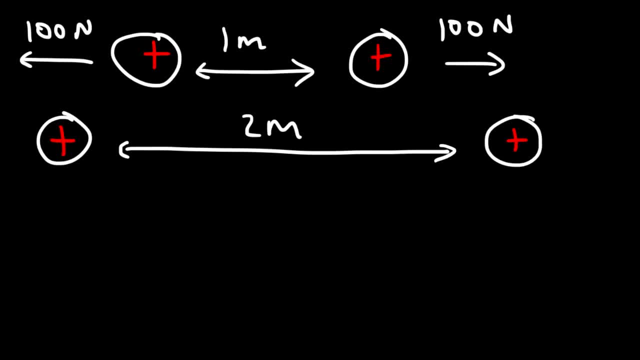 from each other, we expect that the force that's acting on them will be weaker, And so anytime you increase the distance between the two charges, the charge will increase. If you increase the separation distance, the electrostatic force acting on these charges will decrease. 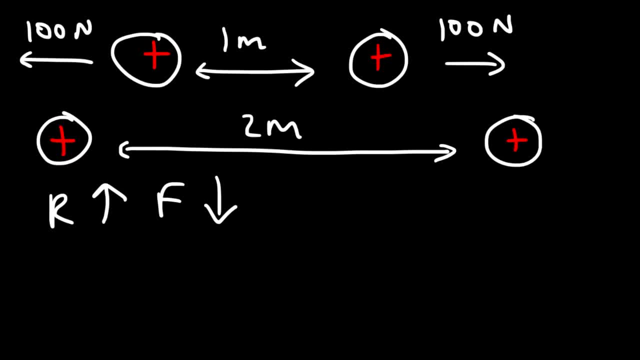 You can liken this to a relationship: When you're close to each other, the bond is stronger, But when you're further away, the bond is weaker, And the same is true for charges: Whenever you have two electric charges that are very close in distance to each other. 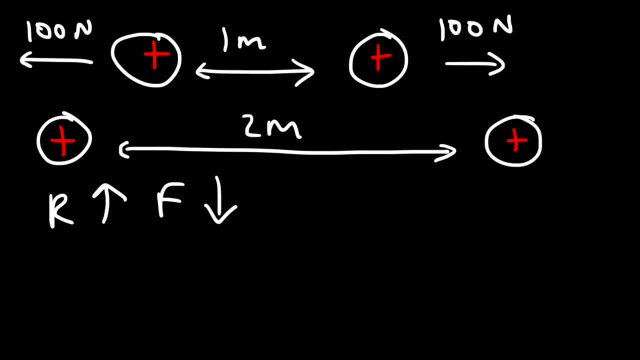 the forces acting on those charges will be strong, Whereas if they're far apart from each other, the forces acting on them will be weak. Now, if we double the distance, what's going to happen to the magnitude of the force? So, using Coulomb's Law, here's what you can do For these types of questions, for any. 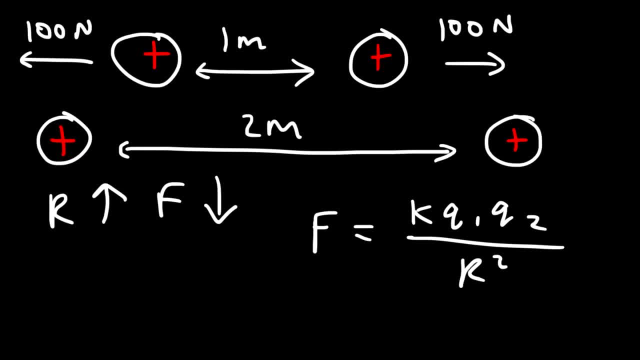 variable that doesn't change or any constant that doesn't change, replace it with a 1. Except for the one that changes. So k, q1, and q2 are not changing in this case, So I'm going to replace it with a 1.. 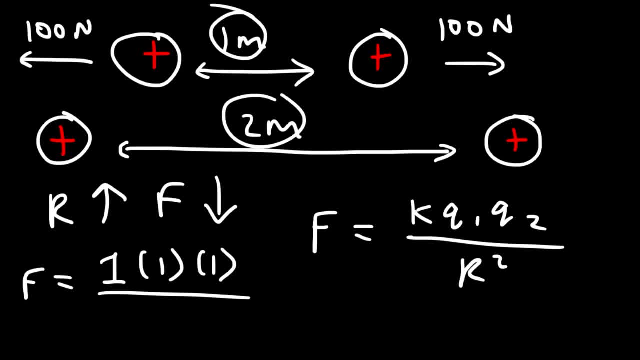 Now the distance increased by a factor of 2.. And so I'm going to replace r with 2.. But because r is squared, I need to square the 2. And 2 squared is 4.. So the force is going to be 1 fourth of what it was before. 1 fourth of 100 is 25.. 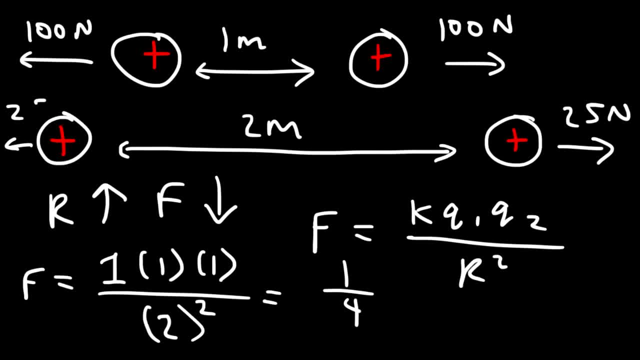 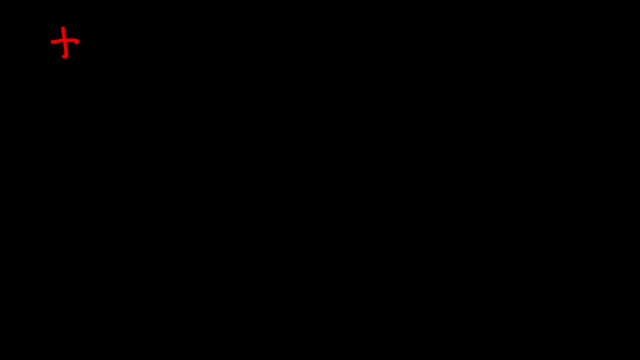 So now the force acting on each charge is 25 N. Now let's say we have a positive charge and a negative charge, separated from each other by a distance of 3 meters. We'll call these q1, and q2.. Now let's say the force acting. 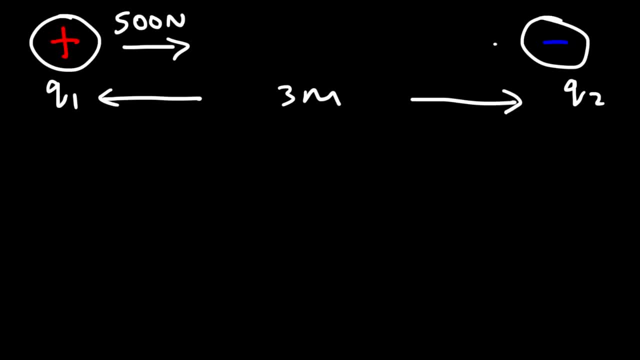 on each charge is 500.. So that will be 0.. Now we'll call this the h. This is 0.. The distance is 2.. So the force is 1.. This is 1. Newtons. So what's going to happen between the forces acting on those? 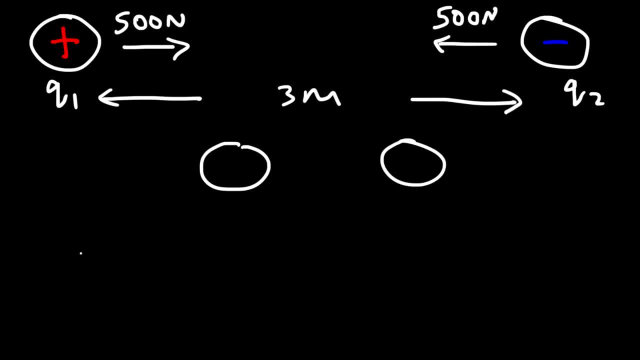 charges if we bring the charges closer to each other. So let's say the separation distance is now one meter instead of three meters. So we reduce the distance by a factor of three, and at the same time let's double the magnitude of charge 1 and let's triple the magnitude on charge 2.. So by 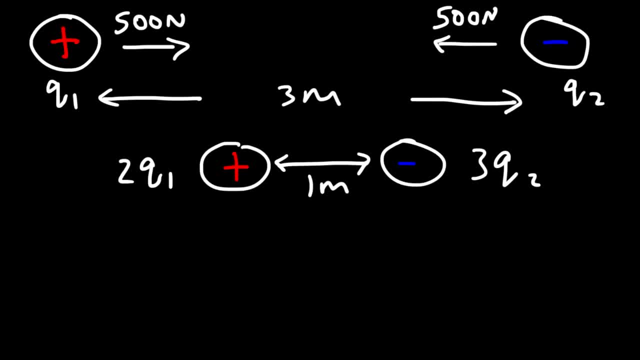 what factor will the force increase by? So, using Coulomb's Law, F is equal to k, Q1, Q2 over R square. The best way to get the answer is to replace everything with the amount that we change it by. Now, k is the same, so let's replace that with a 1.. 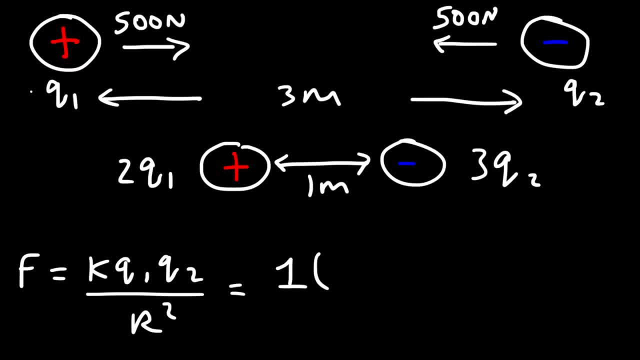 Charge 1. we doubled it and went from 1- Q1 to 2- Q1.. So we doubled Q1.. We tripled Q2 and R was reduced by a factor of three, So it's one-third of its original value and we need to square it. 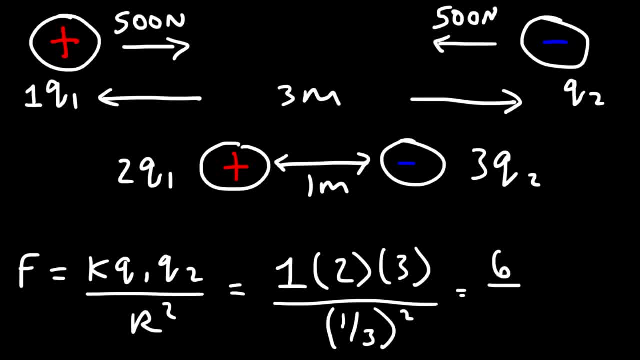 So 2 times 3 is 6.. 1 over 3 squared: 1 squared is 1.. 3 squared is 9.. So this is 6 divided by 1 over 9.. Let's multiply the top and the bottom. 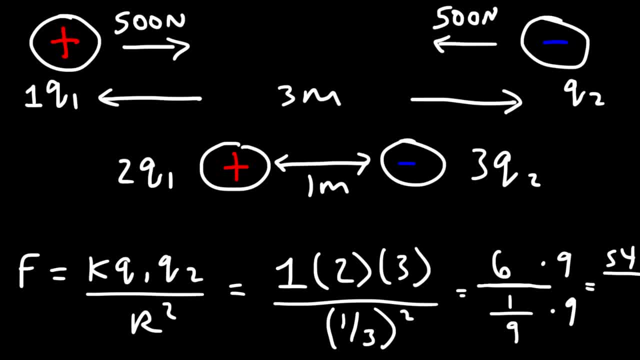 by 9.. 6 times 9 is 54.. 1 over 9 times 9 is 1.. The 9's cancel, So the force will increase by a factor of 54.. Now the original force was 500.. So the new force 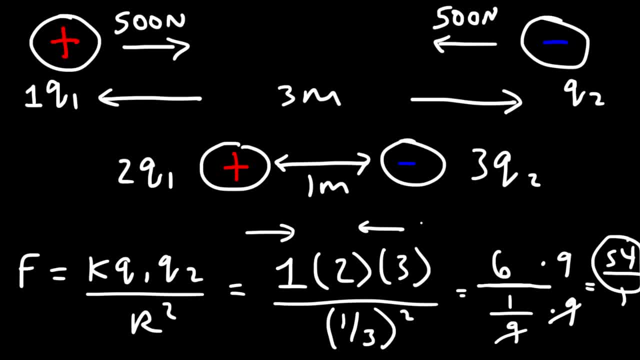 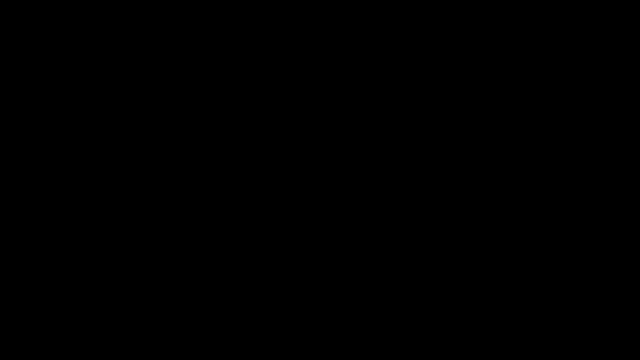 acting on these two charges is going to be 500 times 54, which is 27,000 Newtons. So to review, make sure you understand this: between charges: If you increase the magnitude of the charge, the electrostatic force acting on them will. 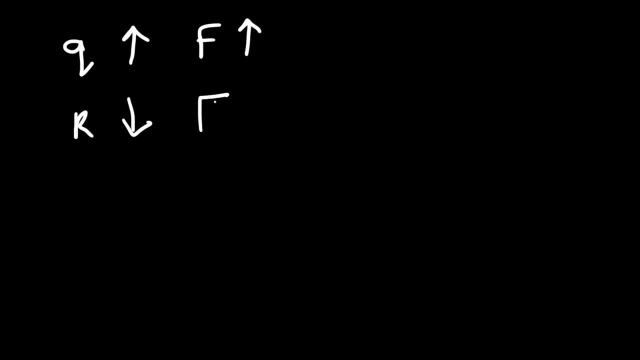 increase. If you decrease the distance, the electrostatic force will increase. Now let's work on a simple math problem relating to Coulomb's law. So let's say that Q1, X, Y is: 1. has a magnitude of 200 microcoulombs and Q2 has a magnitude of 300 microcoulombs. 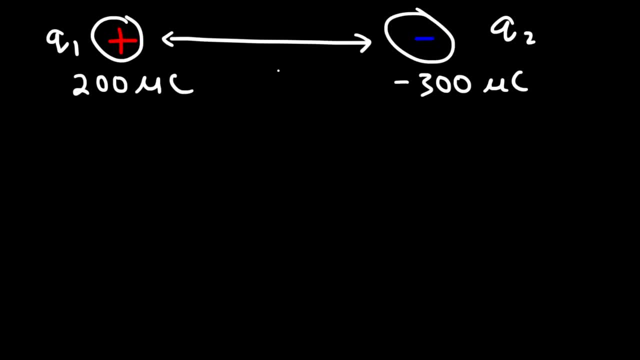 Now, let's say the separation distance between the two charges is 80 centimeters. Calculate the magnitude of the force between them. So we could use this equation: F is equal to KQ1Q2 over R squared. Feel free to pause the video and try this. So K is 9 times 10 to the 9.. 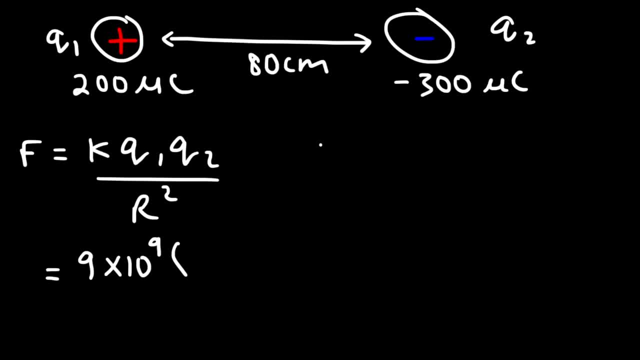 Q1 is in microcoulombs. Micro is 10 to the negative 6.. So 200 microcoulombs is going to be 200 times 10 to the minus 6 coulombs. Now for Q2, we don't have to worry about the negative sign. 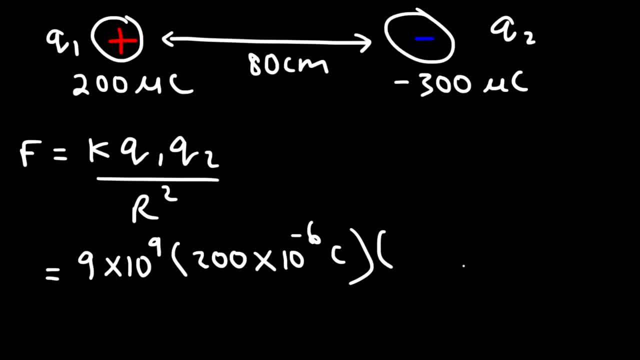 because if you're looking for the magnitude of the force, it's always going to be a positive number. The only thing we need to worry about is the direction. The direction of the force acting on Q1 is going to be towards the negative charge. 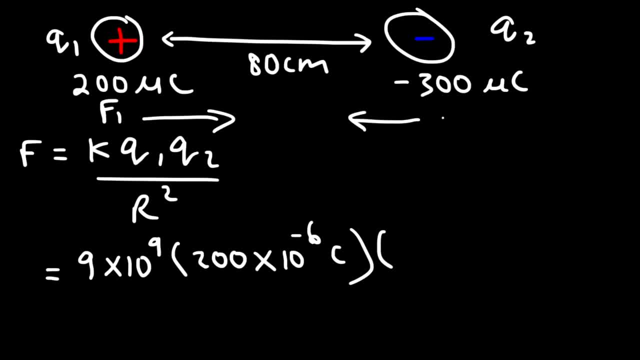 and the direction of the force acting on Q2 is going to be towards the positive charge. So when dealing with opposite charges you're going to have a force of attraction When dealing with like charges, like two positive charges or two negative charges. 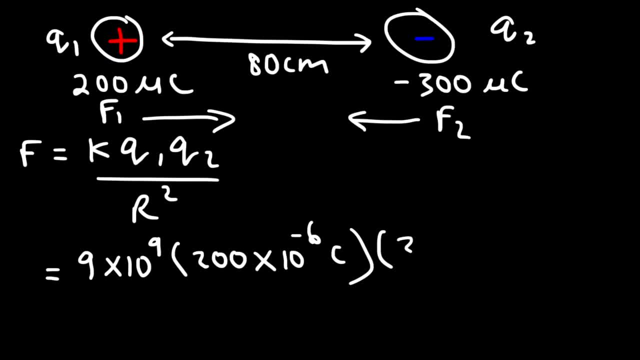 you're going to have a force of repulsion, So Q2, we're going to replace it with 300 times 10 to the minus 6 coulombs. Now the distance between the two charges is 80 centimeters. One centimeter is 10 to the minus 2 meters. 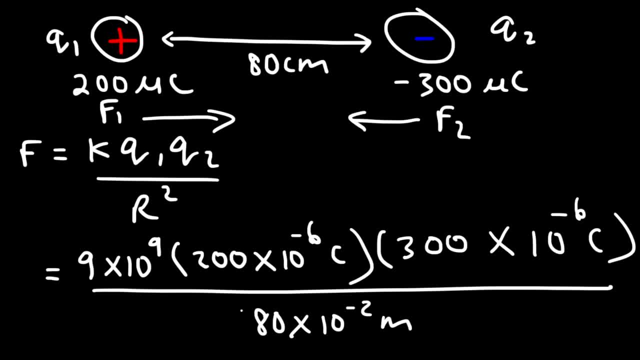 So you can write 80 times 10 to the minus 2 meters, and then we need to square it. So let's go ahead and plug in this whole thing, So you should get 843.75 newtons as the electrostatic force acting on these two charges. 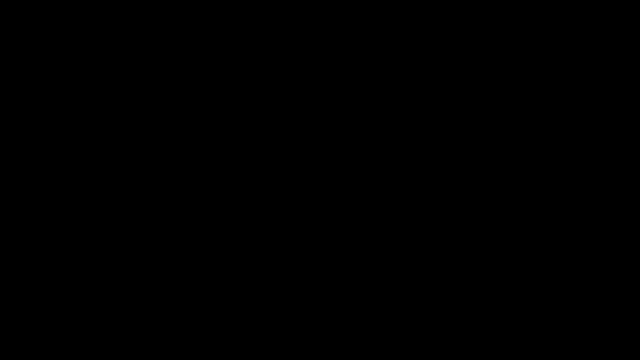 That's the answer. Now you might be wondering what is meant by electric charge. You've heard of that term before and you have an idea of what it is. but what really is electric charge? Q, the symbol for electric charge, represents the quantity of charge. 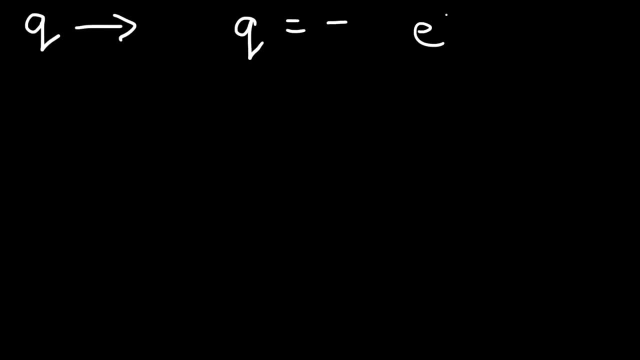 When Q is negative. what this means is that you have more electrons than protons, And when Q is positive, there are more protons than electrons. The charge of one electron is equal to negative 1.6 times 10 to the negative, 19 coulombs. 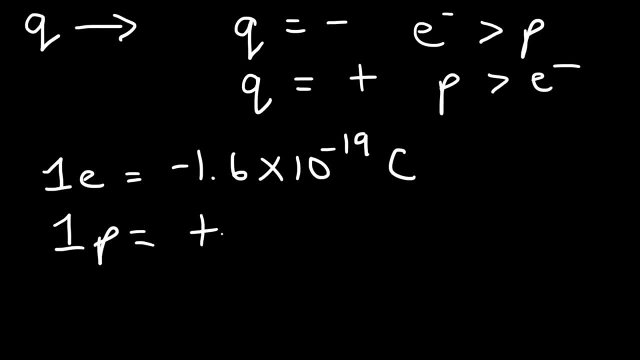 The charge of one proton is equal to: negative: 1.6 times 10 to the negative 19 coulombs. Positive: 1.6 times 10 to the negative 19 coulombs. So let's say, if we have a charge of positive, 100 microcoulombs, 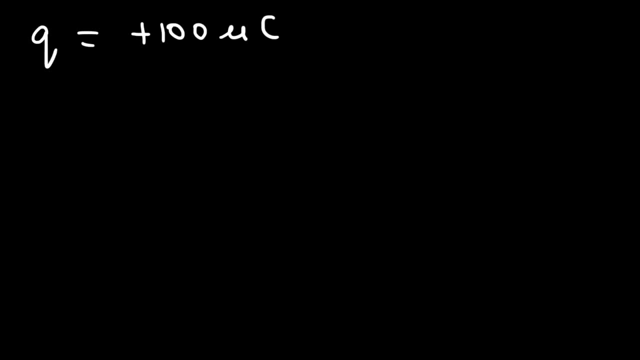 what does that mean in terms of protons and electrons? So using this conversion factor, one proton has a charge of positive 1.6 times 10 to the negative 19 coulombs. 1.6 power contract is comming from one electron to the negative 19 coulombs, not negative 11.. 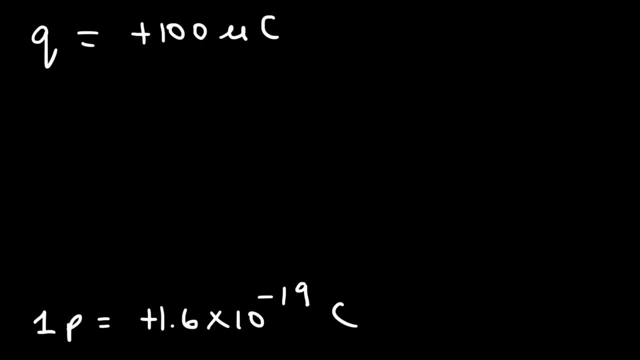 So instead of derivative, we use the conversion factor: determine the number of excess protons that represent this charge. So let's say, if we have a piece of metal with a charge of positive 100 microcouloons, there's more protons than electrons in this object. Now to quantify it, we're. 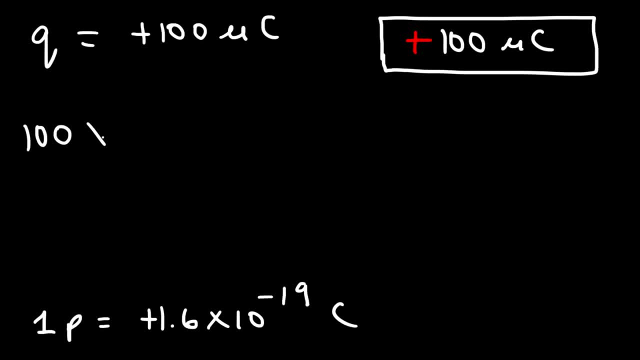 going to convert couloons to protons. 100 microcouloons is 100 times 10 to the negative 6 couloons and we know that one proton has a charge of 1.6 times 10 to the negative 19 couloons. Make sure you set it up in such a way that the unit 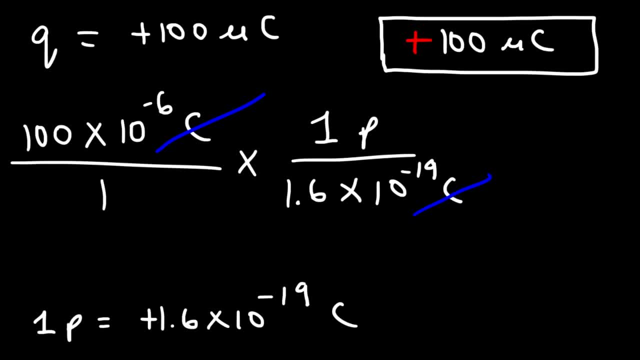 couloons will cancel. So now let's divide 100 times 10 to the minus 6, by 1.6 times 10 to the negative 19, and so the answer is positive: 6.25 microcouloons times 10 to the 14 protons. So what this means is that there's this many protons. 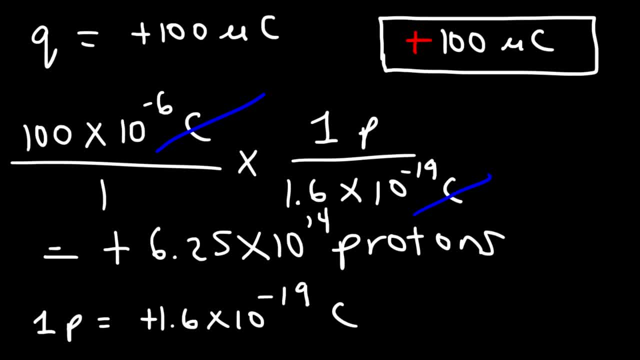 more than electrons. This doesn't tell you how many protons are in the object or in the metal. It simply tells you how many protons or how many excess protons that you have relative to the number of electrons, Because in the metal you're. 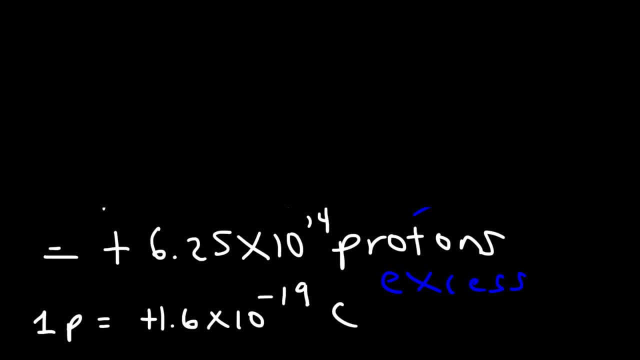 going to have both electrons and protons. So let's say, if there were 1.5 times 10 to the 14 electrons and the objects still have a net charge of positive 100 microcouloons, How many protons will there be? So this number is the difference between the number of 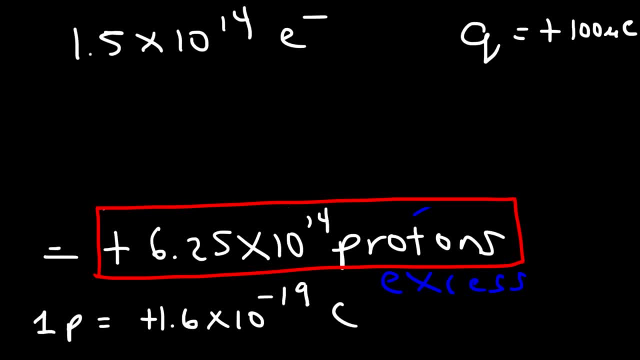 protons and electrons. It just means we have that many more protons than electrons. What we need to do to get the answer is we need to add these two numbers, because there's going to be more protons than electrons. So 1 plus 6 is 7, and 0.5 plus 0.25 is 0.75. 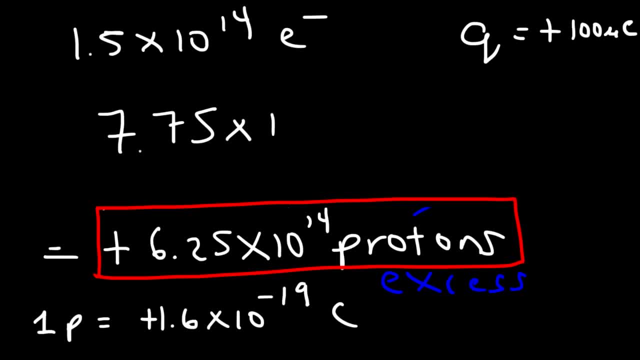 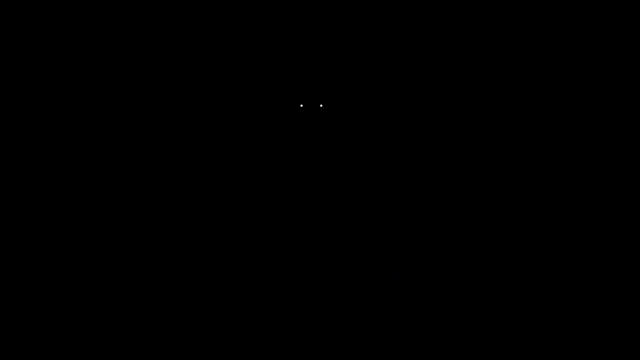 So we're going to have 7.75 times 10 to the 14 protons, And so that's how many protons would actually be present in that object, given this charge? So that's how you could find the answer. Now, let's say, if you have an object with 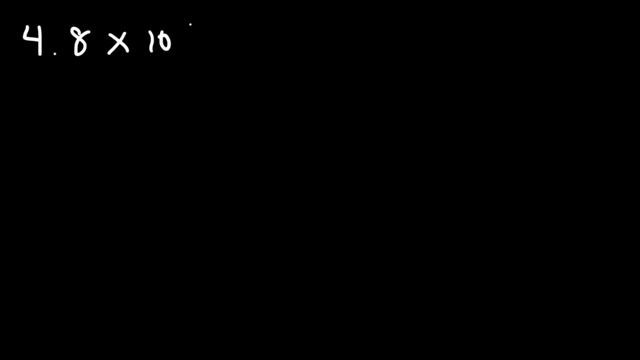 4.8 times 10 to the 16 electrons and it has, let's say, 2.5 times 10 to the 16 protons. So what is the net charge in this object? What would you do to find the answer? 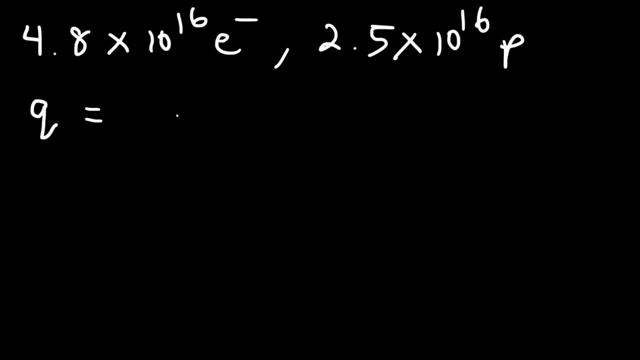 Now there's a simple formula that can help you to calculate the answer: The net electric charge. you could use lowercase q or sometimes capital Q will be used for that. So the net electric charge is going to be the difference between the number of protons and electrons times the individual charge of a proton or an. 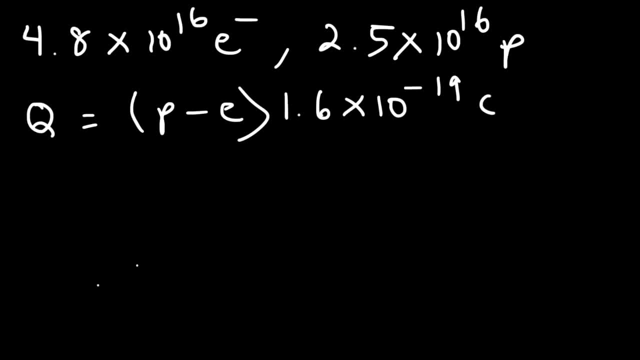 electron. That is the absolute value of that charge, And so that's all you got to do. So in this case, we have 2.5 times 10 to the 16 protons, and we have 4.8 times 10 to the. 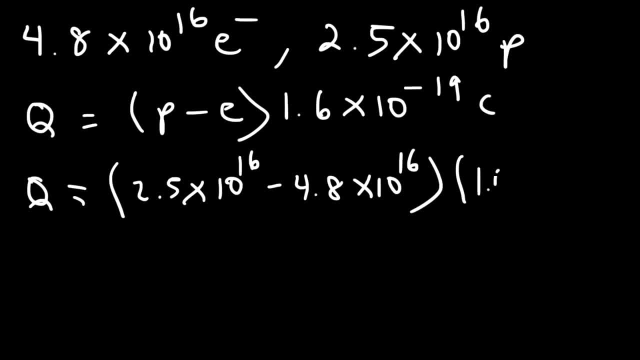 16 electrons. Let's multiply by this number, So 2.5 minus 4.8, that's a negative 2.3.. And it makes sense why it should be negative, because we have more electrons than protons, And so q has. 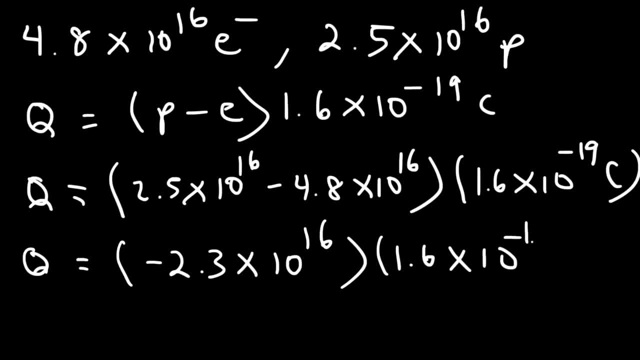 to be equal to a negative number. Now if we multiply these two numbers, this will give us negative 3.68 times 10 to the minus 3 coulombs. Now 10 to the minus 3 is associated with the prefix milli, So we could say that this is negative 3.68 times. 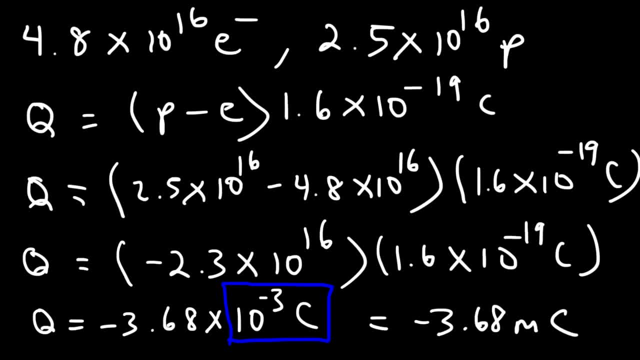 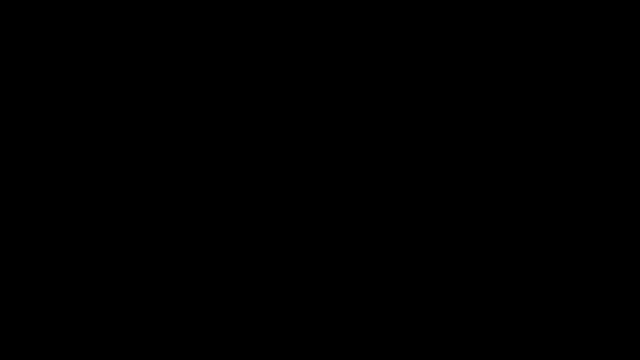 And so we can write the final answer like this: So, as you can see, if you have more electrons than protons, the net charge will be negative. Now let's go back to electric forces, because sometimes you'll be given a situation where 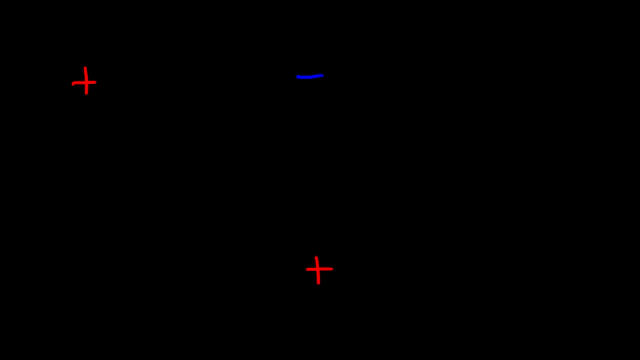 you have multiple charges like this one, But let's focus on the concept more than the math associated with these types of problems. Let's call this Q1,, Q2, and Q3. And here is the question: What is the direction of the net electric force acting on Q2?? 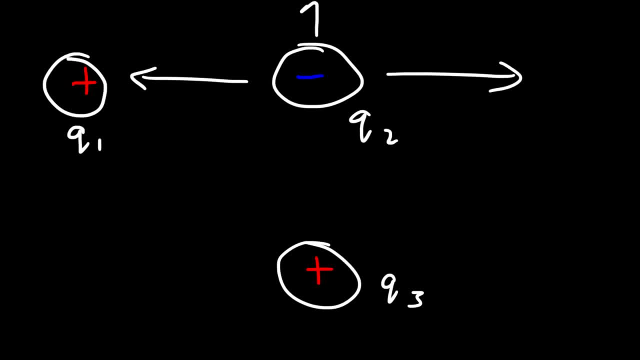 Is it this way? Is it that way? Is it going north? Is it going southeast? Okay, So what is the direction of the net electric force? And let's say that each charge has the same magnitude and all of the charges are equally. 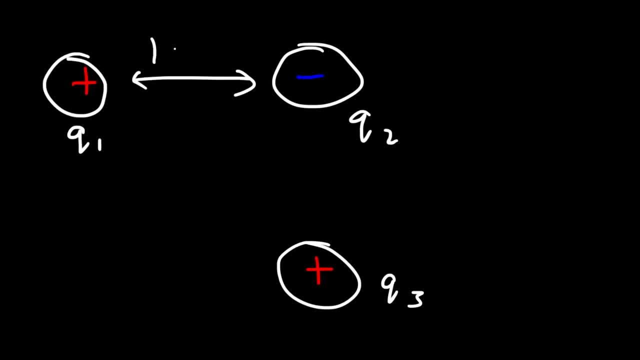 distant from each other. So let's say Q1 and Q2, they're one meter apart, and Q2 and Q3 are also one meter apart. Now, focusing on Q2, Q2 is attracted to Q1. And so Q1 is attracted to Q2.. 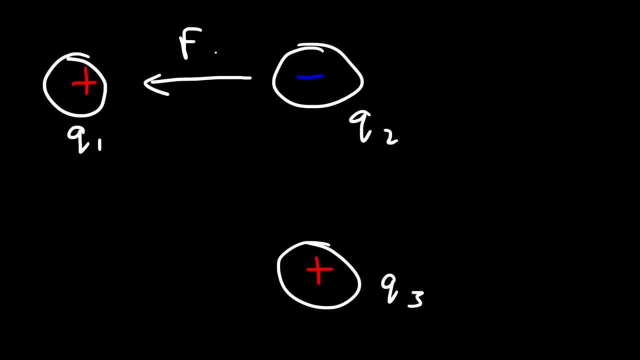 Q2 is attracted to Q1. And so it feels a force that pulls it to the left. Q2 is also attracted to Q3. It feels a force that pushes it down. And so if you combine these two vectors, if you go to the west and also south, the resulting 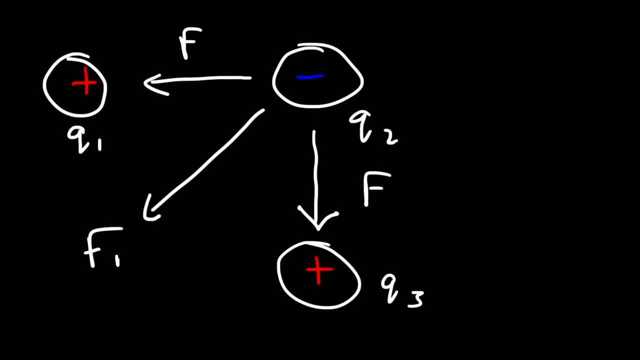 force vector will be directed southwest, And so, at this instant of time, Q2 is going to feel a force that pulls it to the right. So let'sיקoo2, ts-tri, b-2-q3-r2-sk2-pr-x-n-k-n-cimento, ta-n-n. Dragons in theVERTING method. 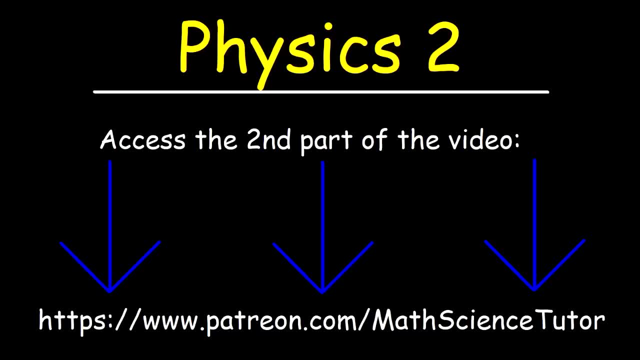 of force that's going to pull it in this general direction. The video that you're currently watching is the first half of the entire video. For those of you who want access to the second part of the video, I'm going to put it on my Patreon. 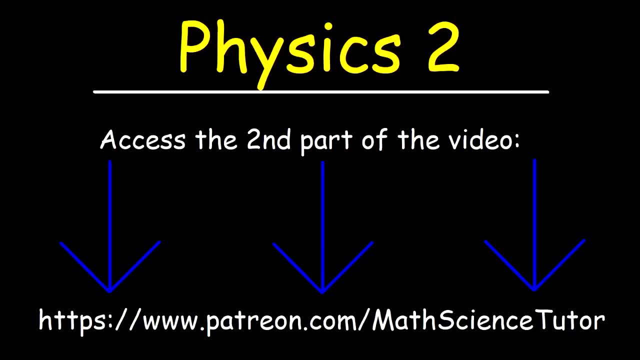 page which you can see the link on the screen, and if you wish to support that page, you can gain access to the second part of the video. Now, in that video, I'm going to talk about capacitors, how they work and some things you need to know. 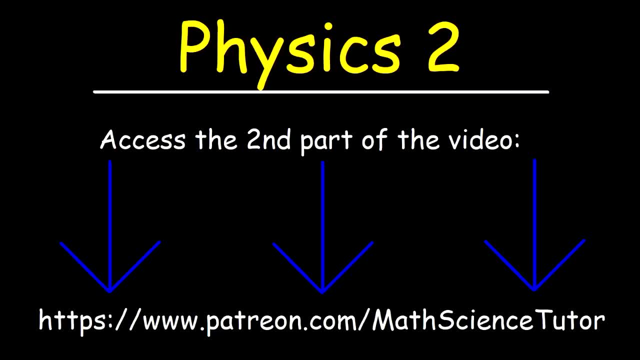 about them. in addition to that, circuits, Ohm's law, Kirchhoff's voltage law, his current law and also a series and parallel resistors and things like that. So feel free to take a look at that video if you want to, and I do have some. 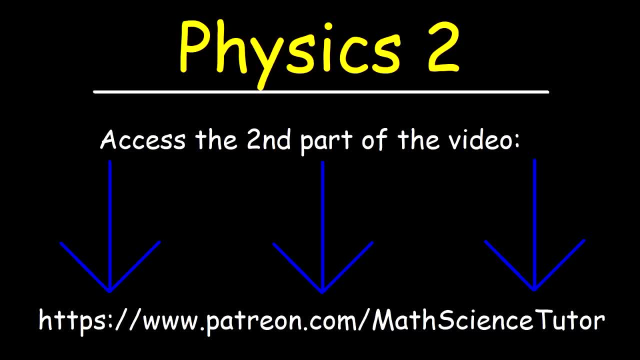 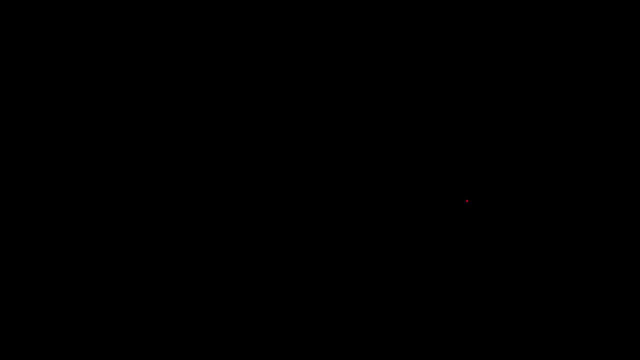 other video content that you might be interested in on my Patreon page. So when you get a chance, feel free to review it. and now let's get back to this video. Now let's try another problem. So let's say that this time we have three positive charges. We'll call it Q1,. 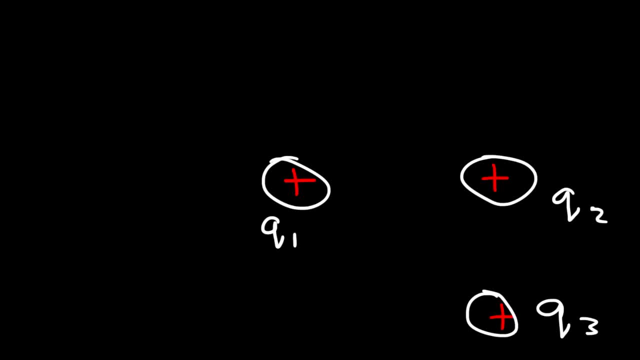 Q2, and Q3.. What is the direction of the net electric force acting on Q1?? Let's say, just like before, the charges have the same magnitude and they're equally spaced apart. What is the direction of the force acting on Q1, or approximate the? 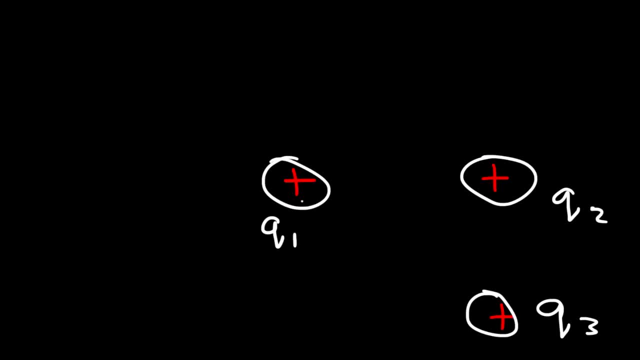 direction. Now Q1 is repelled by Q2, so Q2 causes Q1 to move in this direction. Let's say the distance here is one meter and the distance here is one meter. Now the distance between Q1 and Q3 will be more or greater than one meter, based on: 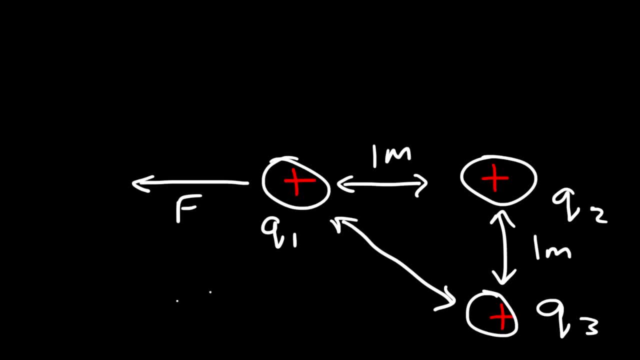 the Pythagorean theorem. So if you basically use C squared equals A squared plus B squared. if you take the square root of 1 squared plus 1 squared, you're going to get the square root of 2, which is about 1.4.. And so, because the distance between Q1 and Q3 is greater, 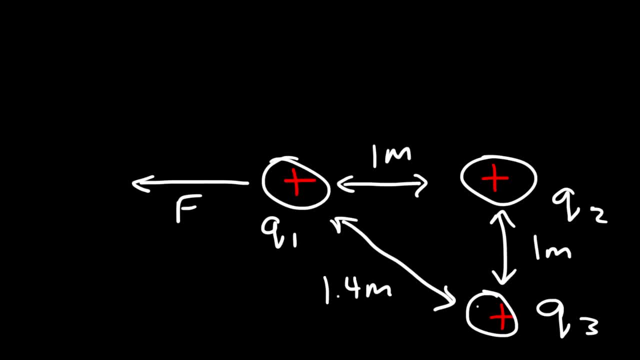 than that between Q1 and Q2, the force that is exerted on Q1 by Q3 is going to be weaker than this force, But this force will be in this direction. but we should draw a smaller vector, So I'm just gonna make that vector smaller. Now, if we were to combine these, 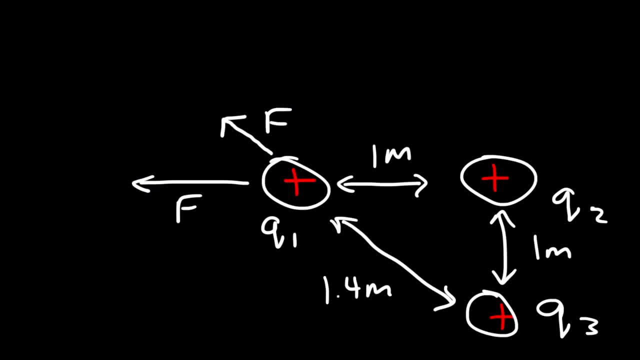 two vectors, what would we get? One way to add vectors graphically is to draw them from head to toe. So if we draw the first vector, which is going to be longer, let's call this F2, because it was based on charge 2.. 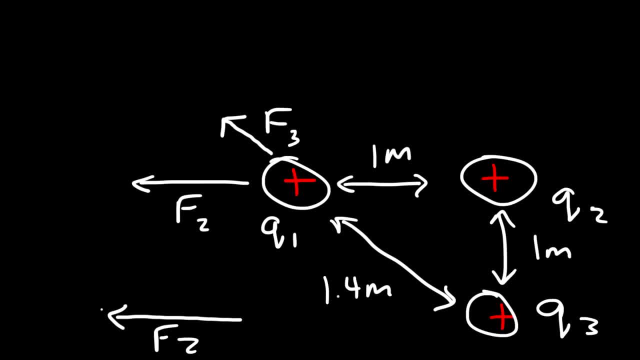 We'll call this F3.. And then the second vector, which is going in this general direction, but it's shorter, And then, starting from the original position to the final position, this would be the resulting vector. We'll call it FR. 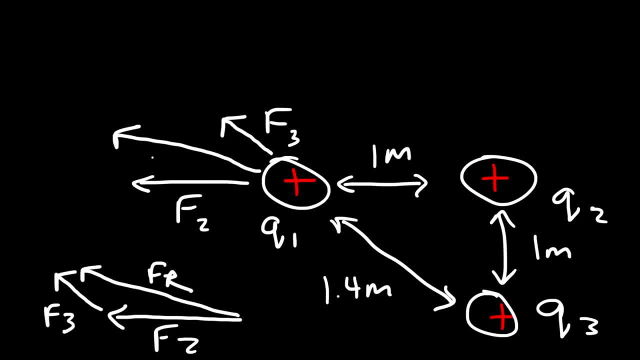 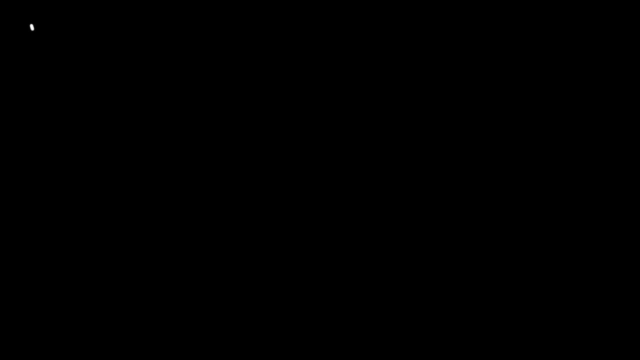 So it looks something like this: So that's going to be approximately the direction of the resultant electric force acting on Q1. And so that is our answer. Now let's talk about something known as the electric field. This is the next topic beyond electric force. 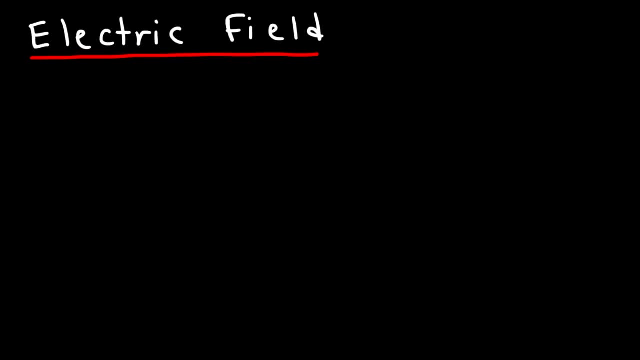 So what is the electric field? The electric field is defined as the force exerted on a positive test charge divided by the magnitude of that test charge. And so here's the formula for the electric field: It's equal to force divided by charge. So let's say: 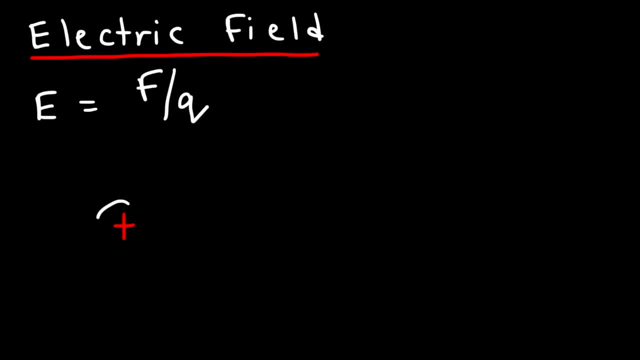 if we have a positive charge, and let's say this positive charge has a magnitude of 50 microcouplems and it feels a force that pushes it towards the right, And let's say the magnitude of that force is 0.02 newtons. What is the electric field? 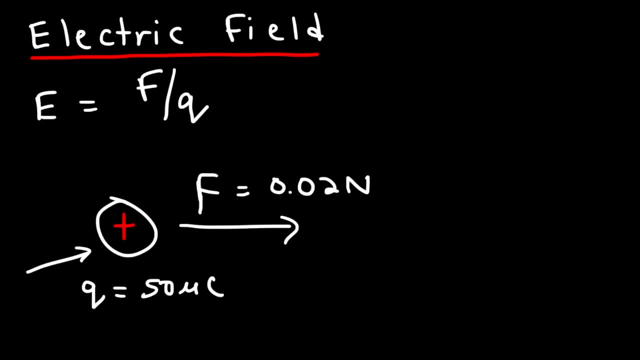 at that point in space. So using this formula, it's simply the force exerted on a charge divided by the magnitude of that charge. So it's 0.02 newtons divided by 50 times 10 to the minus 6 coulombs. 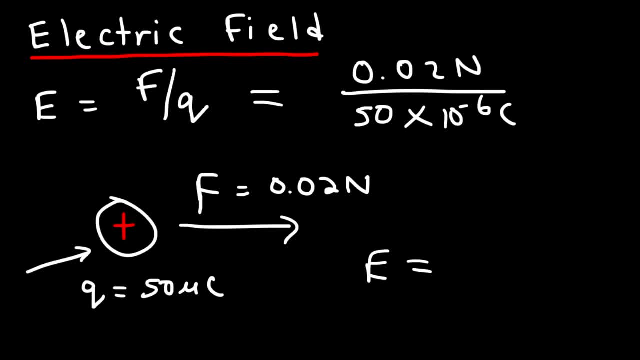 So the electric field in this region of space which the positive charge currently occupies, the electric field in that region is 400 newtons per coulomb, And so the electric field is basically the ratio between the force exerted on a charge divided by the 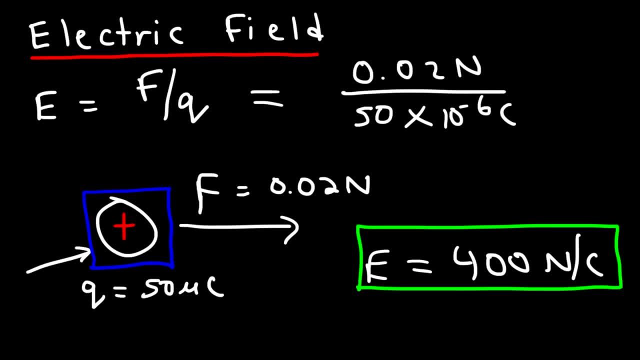 magnitude of that charge. So think about what this number means. So this electric field tells us that at that point it can exert a force of 400 newtons per every coulomb of charge. So if you have a charge of one coulomb, so let's say this is a. 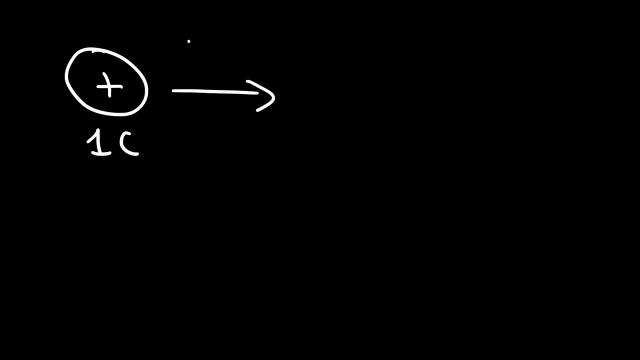 positive charge of one coulomb, it will exert a force of 400 newtons. Now if we double the magnitude of the charge, but the electric field is still the same, that is 400 newtons per coulomb the force. 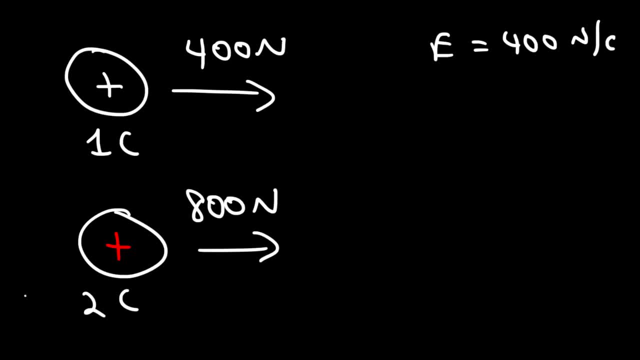 exerted on that charge will be 800. And so as the magnitude of the charge increases, the force that's exerted on that charge by the electric field will increase, And so the electric field gives you a ratio between how much force will be exerted per unit of charge. So if we 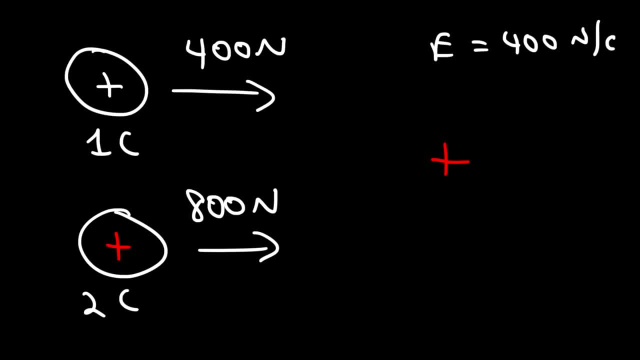 have, let's say, another positive charge. with a charge of five coulombs, the force exerted on it will be 5 times 400, and so it's going to be 2,000 newtons. So let's say that we have an electric field. 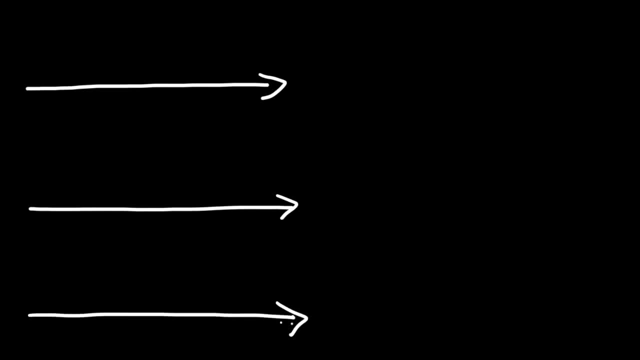 vector that is directed east. What's going to happen if we place a positive charge in this electric field? Let's compare it if we place a negative charge in that same electric field. So what you need to know is that a positive charge will fill a force in the same direction. 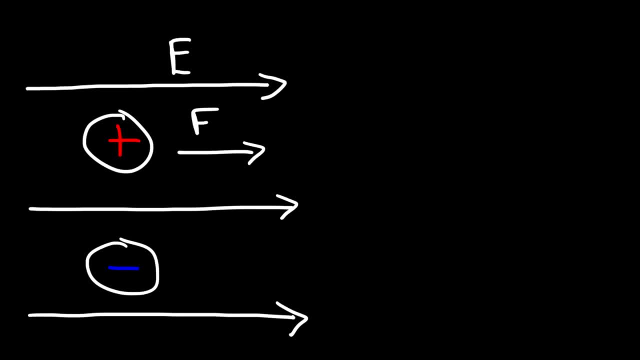 as the electric field. A negative charge will fill a force that will accelerate it in the opposite direction of an electric field. So let's say, if we have an electric field directed north, So go ahead and draw the direction of the electric force acting on these two. 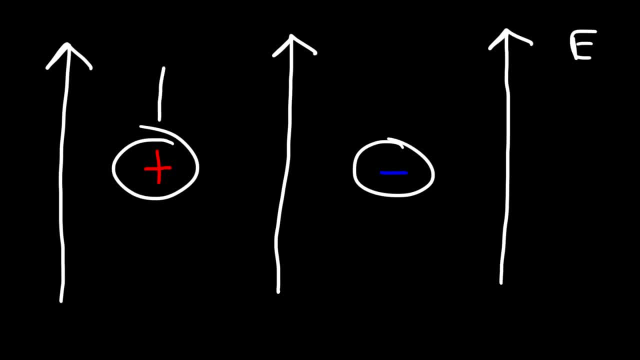 charges. So the electric force acting on the positive charge will be directed north, in the same direction as the electric field. For the negative charge, the electric force will be directed south, opposite to the direction of the electric field. Now it's important to 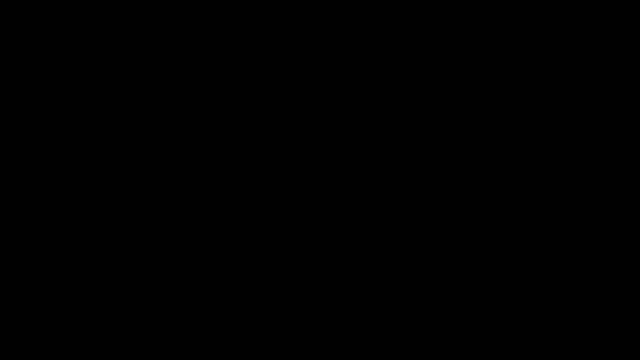 understand that every charge can create its own electric field. The electric field created by a positive charge emanates in all directions away from the positive charge. Now, the electric field created by a negative charge always points towards the negative charge. Now, why is this important to know? 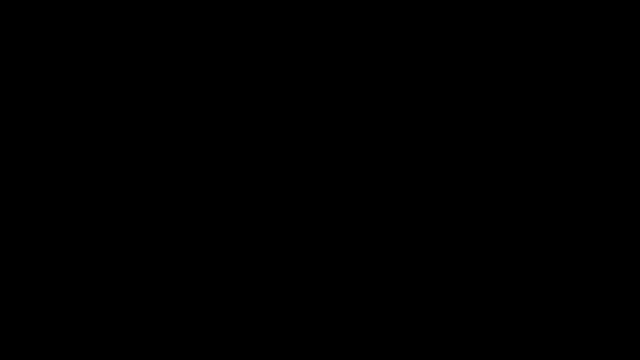 Sometimes you might be given a situation where you have multiple charges. Let's say: let's start with a simple situation. Let's say we have a positive charge and a negative charge and we wish to determine the direction of the electric field at three points. 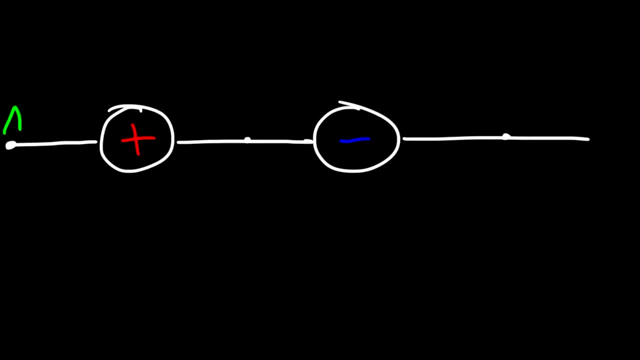 Let's say at point A, at point B, which is at the midpoint between Q1 and Q2, and also at point C, What is the direction of the electric field at these points? Well, let's start with point B, So to 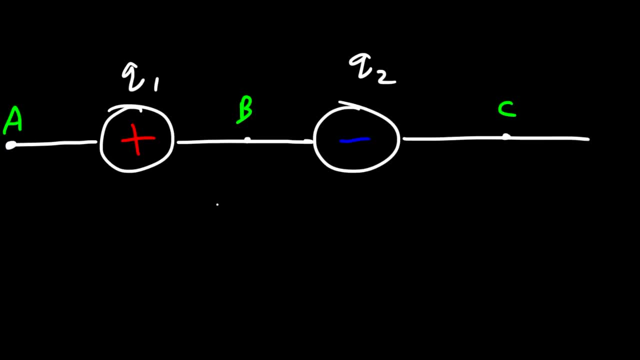 determine the electric field exerted by Q1 at point B. draw a line from Q1 to point B. We'll call this E1. Because it was created by Q1.. Now to draw the electric field vector created by Q2 at point B- remember from a negative. 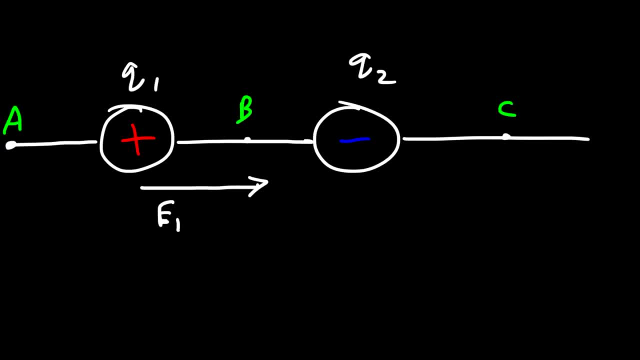 charge. the electric field created by it has to go towards the negative charge. So E2 will be a vector starting from point B, drawn to the negative charge. So it will be in this direction. So at point B the net electric field will be directed east. 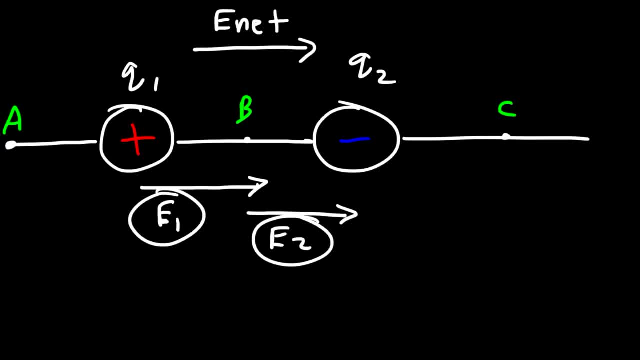 Because it's the sum of these two vectors. Now let's focus on point A. The electric field at point A, created by Q1, will be in this direction, So this is going to be E1.. So you need to draw it from the positive charge to the point. So 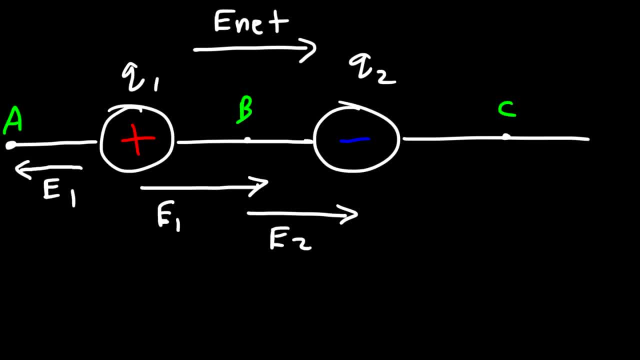 remember, the electric field created by any positive charge always emanates away from the positive charge. Now, the electric field created by Q2 at point A, because it's a negative charge, we need to draw it from the point pointing towards a negative charge. Now this: 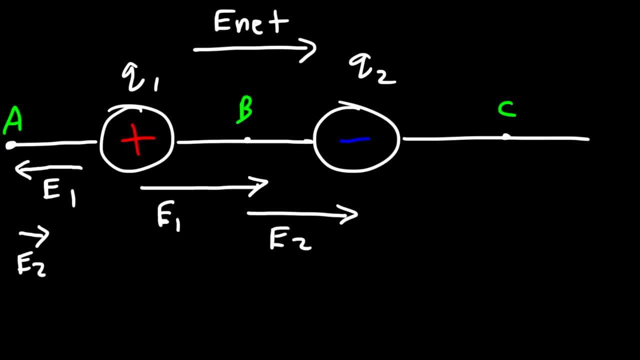 vector is going to be smaller than E1.. And the reason why E2 is smaller than E1 is because E2, I mean Q2, is further away from point A than Q1, is Because Q1 is closer the electric field created by Q1. 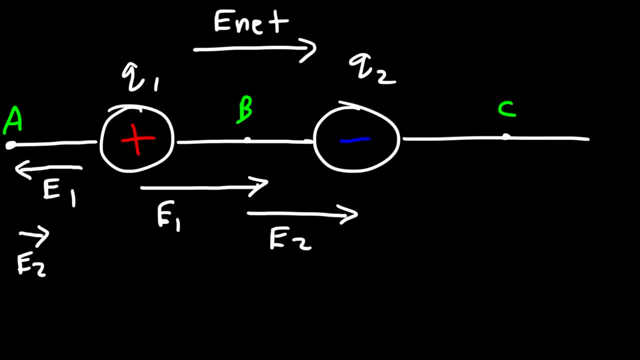 is going to be stronger than Q2.. So the electric field created by Q1 is going to be stronger than Q2.. So here's the formula for the electric field created by charge: It's KQ over R, squared As you increase the magnitude of. 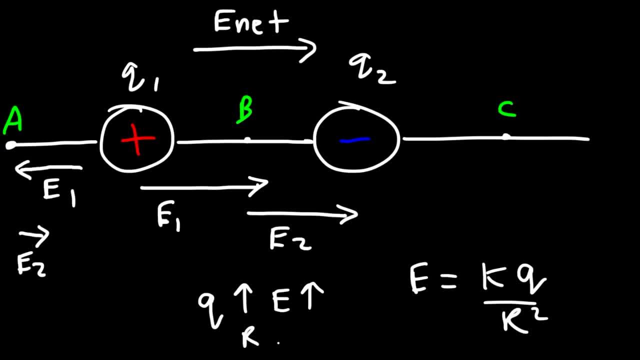 the charge, the electric field increases. As you increase the distance, the electric field decreases And that's why E2 is less than E1 at point A. It's because the distance between Q2 and A is greater than the distance between Q1. 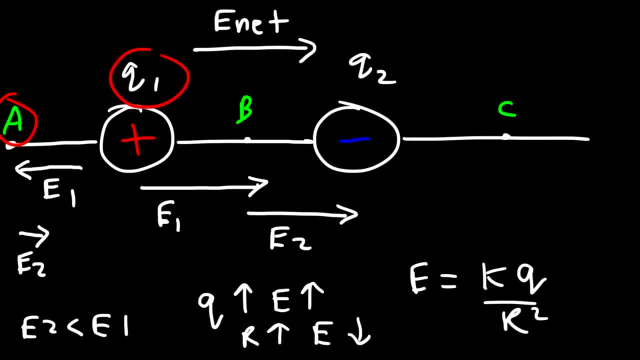 and A, And so that's why Q1 is stronger. I mean, E1 is stronger but E2 is weaker. So the net electric field at point A is going to be directed west as opposed to east, because E1 is greater than E2.. Now 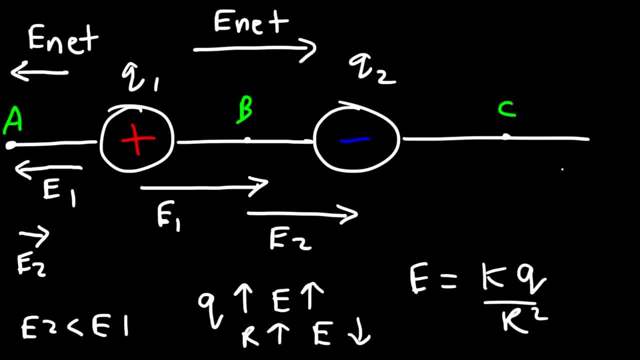 at point C to draw E1, it's going to emanate away from the positive charge towards point C, So it's going to be going in this direction. And for E2, it's going to point towards the positive, I mean towards Q2,. 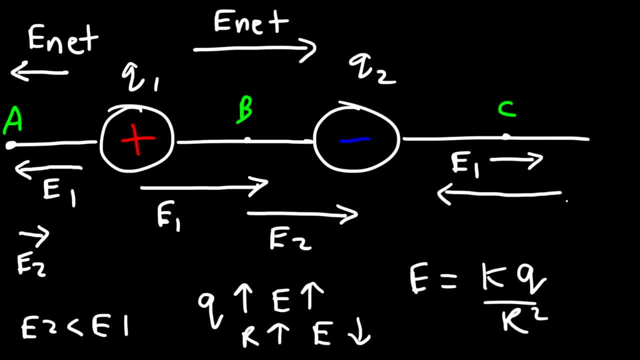 that is, towards the negative charge, And it's going to be bigger because point C is closer to Q2 than it is to Q1. So this time E2 is greater than E1. And so the net electric field will be directed west again because this vector 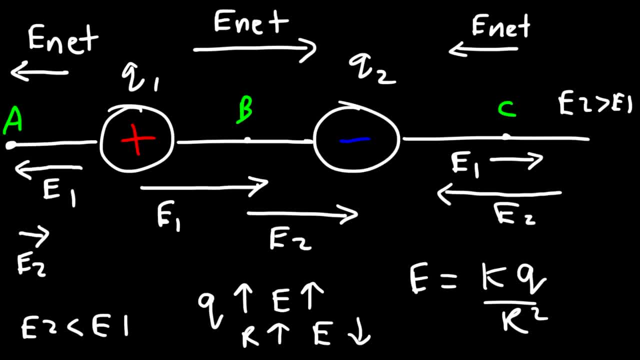 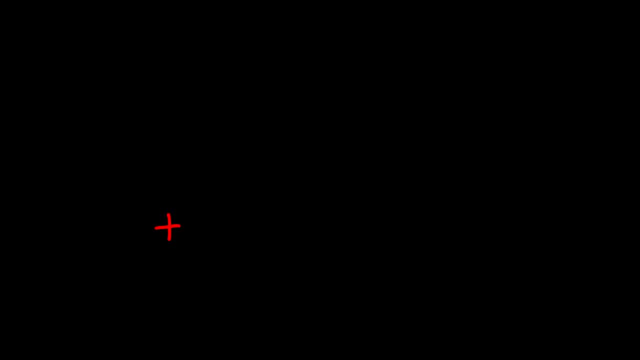 is bigger than this one, And so that's how you could determine the net electric field at a certain point if you have multiple charges. Now, let's say if we have a positive charge in this region and a negative charge here, And so let's. 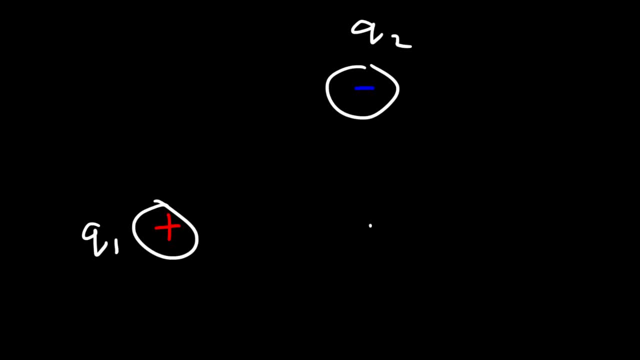 call this Q1 and Q2.. What is the direction of the net electric field acting at point A? So feel free to pause the video, Draw the vectors and determine the net electric field vector at point A. So Q1 is going to exert an electric 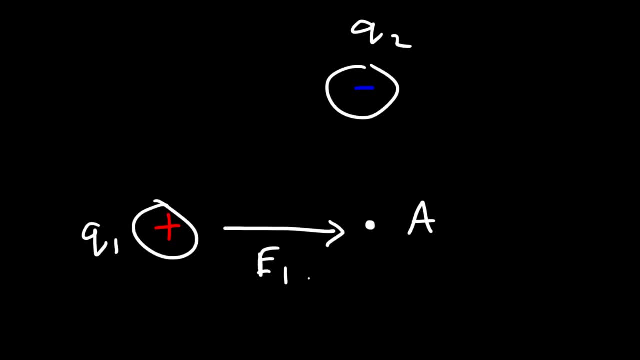 field in this direction, towards point A, Q2 is going to exert an electric field toward itself from point A in this direction. So if we add those two vectors, the resulting vector, so we have E1 going in this direction and then E2, so the resulting vector is: 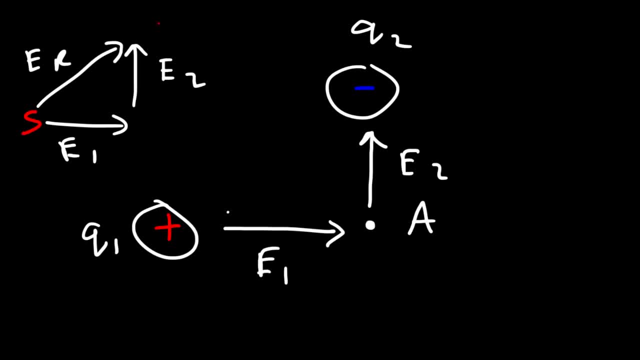 here. So this is where we started and this is where we finished. So at point A the net electric field is going in this direction, So it's going in a northeast direction. Let's try another problem. So let's say we have three charges. 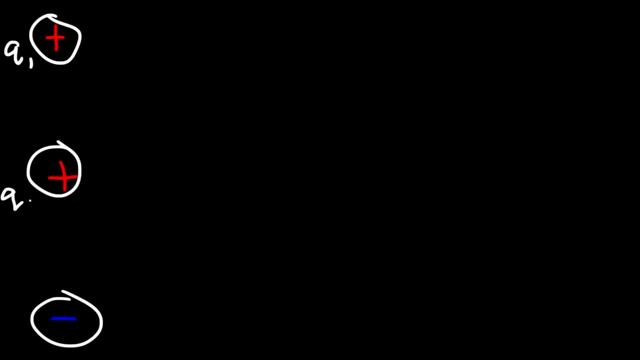 Let's say Q1, Q2, and Q3.. And let's say that they're equally spaced apart. So let's say the distance between Q1 and Q2 is one meter, and the same is true between Q2 and Q3. 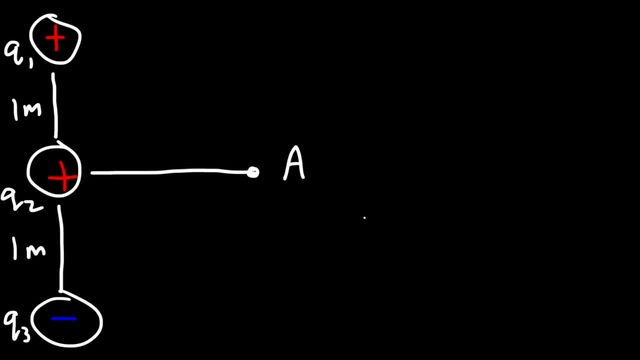 What is the net electric field at point A? What is the direction of the net electric field at that point? So Q1 is going to exert an electric field away from itself towards point A, and the same is true for Q2.. Positive charges always. 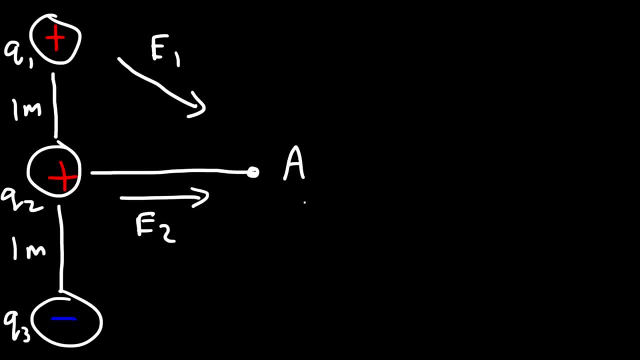 direct an electric field away from them, and the electric field will always points toward the negative charge. And so these are the three vectors that we have, And all the charges have the same magnitude. And so E1 and E3, they're going to be the 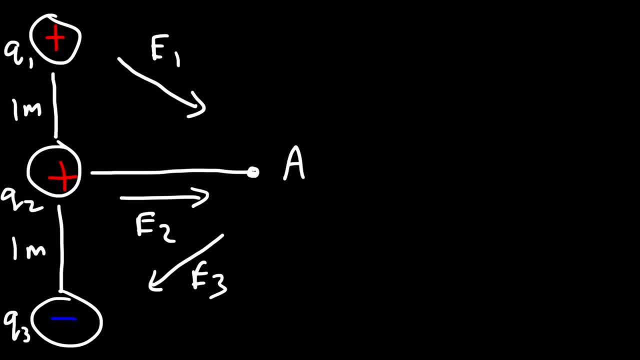 same length. However, E2 should actually be the biggest In terms of distances. let's say that the distance between Q2 and A is one meter. This is going to be about 1.4 meters, and this is going to be 1.4. 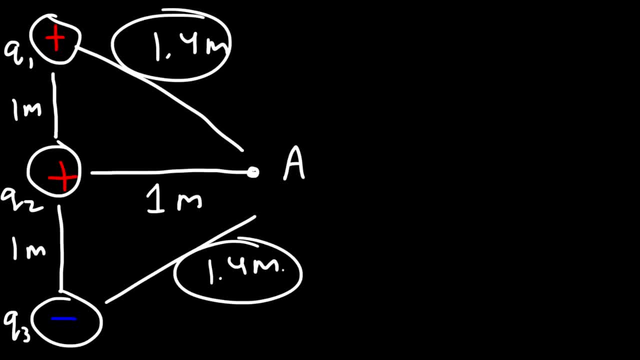 meters. So the electric field vectors for those two should be the same, But this one, because the distance is the shortest, it's going to have the greatest electric field. So E2 is greater than E1 in terms of magnitude, and E1 and E3, they 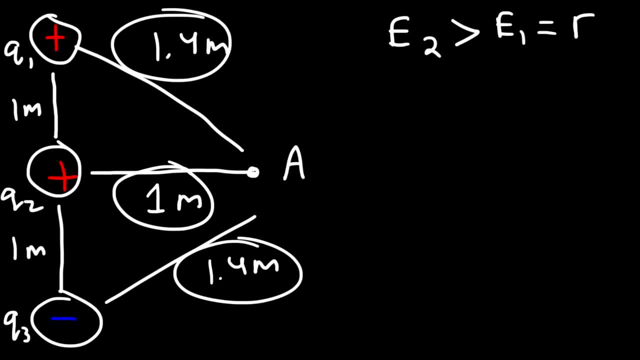 have the same magnitude. So that's going to give us- let me just delete this first. that's going to give us a good idea of how long we should draw the relative vectors E2 is greater than E1 and E1 is equal to. 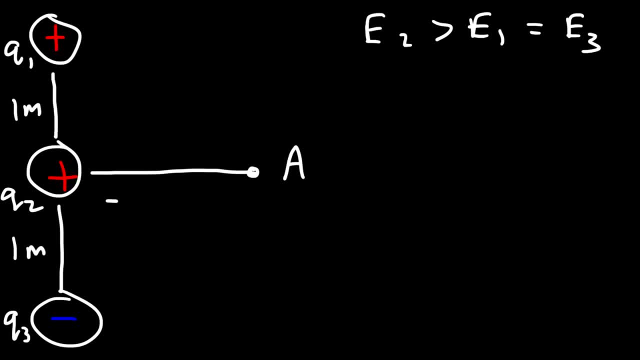 E3. So we're going to say that E2 is about that long, E1 is going to have to be shorter and E3 will also be shorter, but the same length as E1. So how can we add these three vectors so that we can? 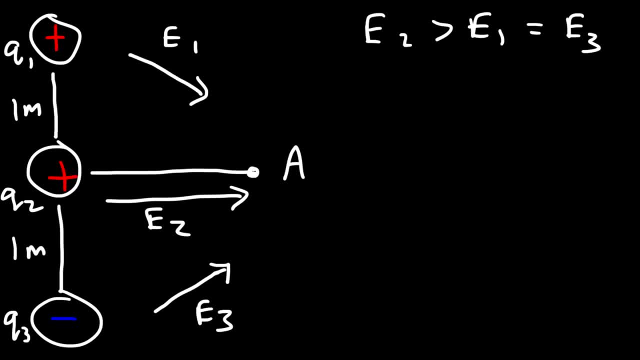 get a general idea of the direction of the net electric field at point A. Now what we need to do is break up E1 and E3 into its components. So E1 has a y-component that is going in the negative y direction and E2 has an. 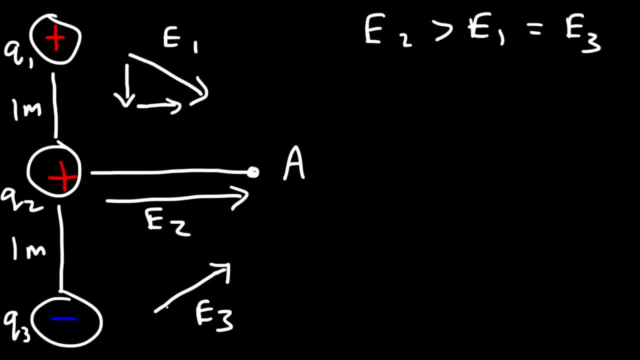 x-component that's going in a positive x direction. E3 has a y-component going up and an x-component going in that direction. Actually, I need to correct this. E3 should be going towards the negative charge. So correction: I had it before but for some reason I had it pointing towards A. 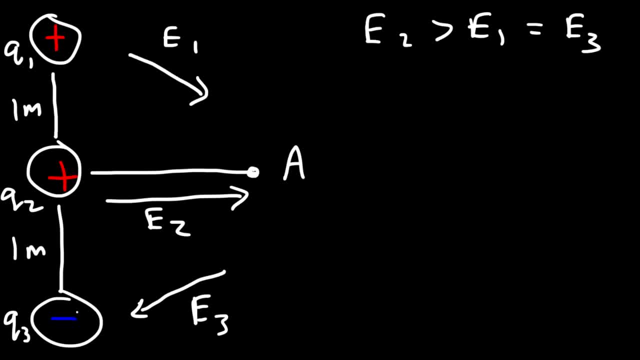 But the electric field created by a negative charge should always point towards a negative charge. So E1 still has a Y component going in a negative Y direction and a positive X component. Now E3 has a negative X component and a negative Y component. 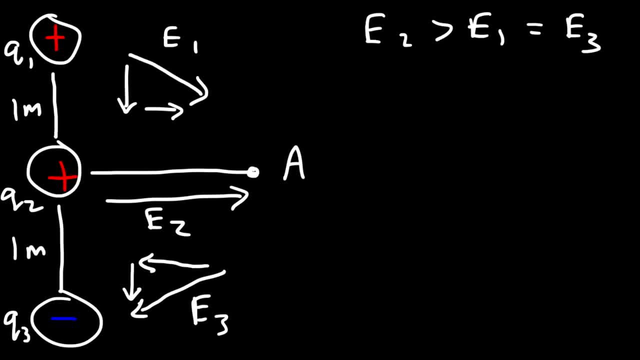 Now, because E1 and E3 are of the same magnitude, we could say that the X component of E1 and the Y component- I mean the X component of E3, they cancel because they're anti-parallel and they're the same length. 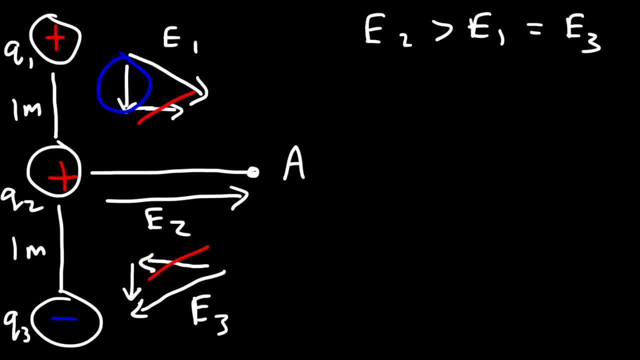 So we could cancel those two. Now notice that the Y components: they're parallel, They're going in the same direction, And so we can add those two Y components to form a bigger vector going in the Y direction, Which I'm going to draw in blue. 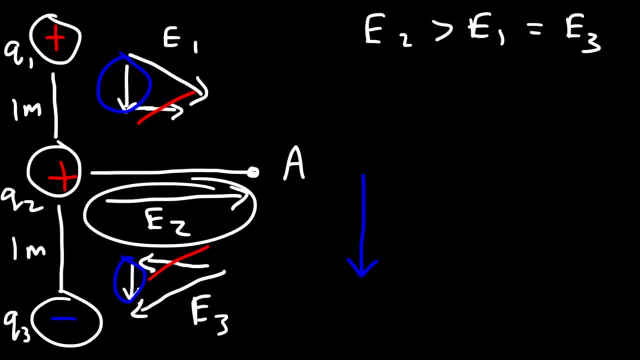 And now let's combine that with E2, which is going in this direction, And so the net electric field. if we combine these two vectors- or let's delete this one and just add it here- we can see that the net electric field is going to be in that direction. 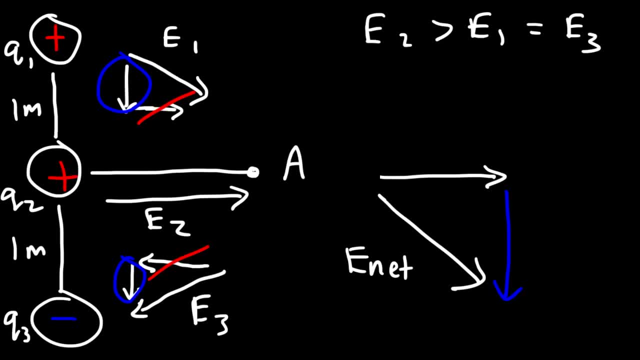 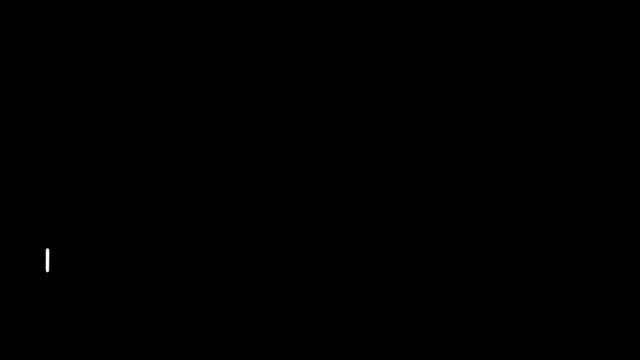 And so that's how you could determine the net electric field vector for this particular problem. Let's say, if we have two charged metal plates, On the left side, this plate will be positively charged And on the right side this will be negatively charged. 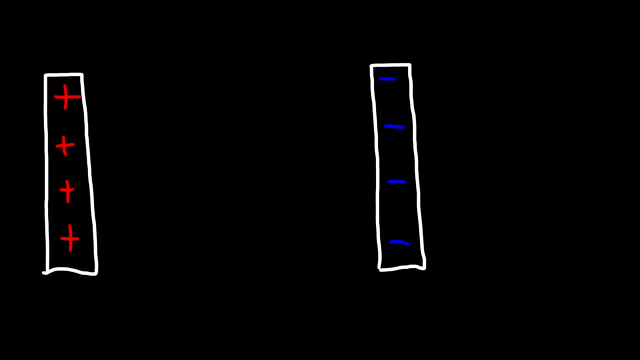 They are positively charged. Now what's going to happen if we place a positive charge near the positive plate? What's going to happen Now? there is an electric field in between the two plates. We know the electric field emanates away from the positive plate and points towards the negative plate. 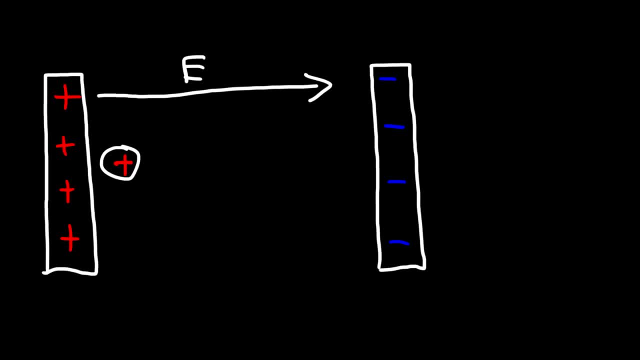 If you recall, positive charges create an electric field that emanate away from them and negative charges create an electric field, and all their cases close to each. otherwise that points towards them. So the net electric field in between these two plates is directed towards the negative plate. Now the positive charge will feel. 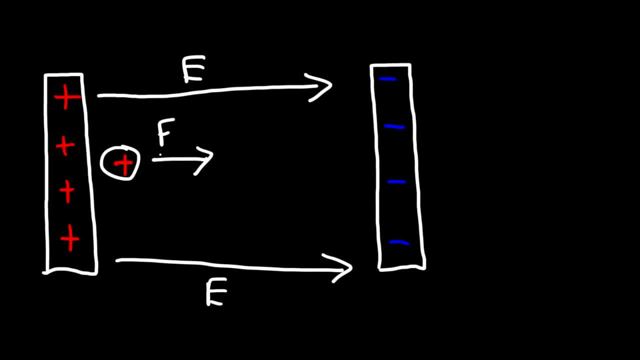 a force that will accelerate it in the direction of the electric field. Now, this electric field, would you say it's doing positive work or negative work. on the charge, Let's say the charge was initially at rest at point A and it's moving to point B. In this case the work done is positive. If you recall, work is. 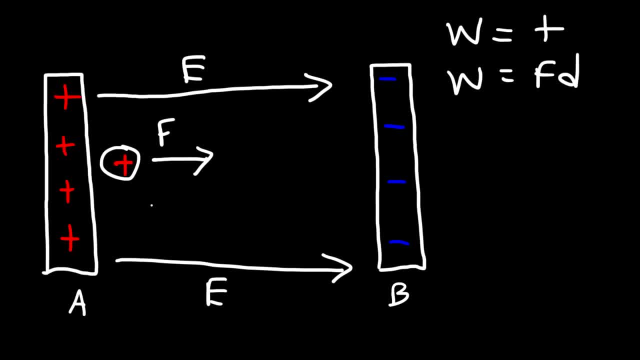 equal to force times displacement. Because the charge is moving to the right, its displacement vector is towards the right. If the force and displacement vector are parallel, then the work done is positive. Because the work done is positive, the kinetic energy of the object is increasing. 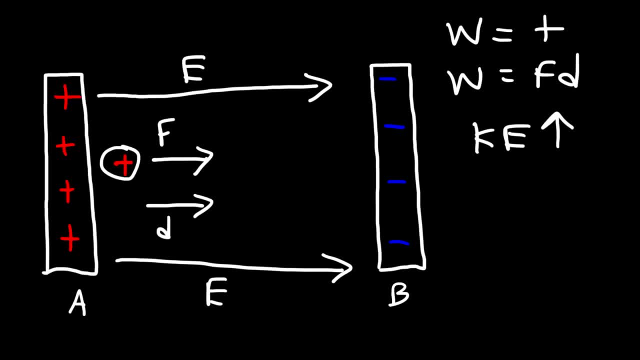 And also the fact that the object is speeding up, It's moving from rest and it's accelerating towards the right. So anytime the speed of an object increases, the kinetic energy increases. And if the kinetic energy increases, that means that the potential energy must be decreasing. 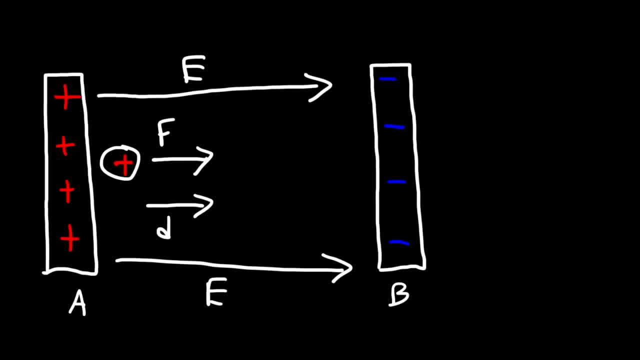 Now let's say, if the positive charge is placed towards the middle or somewhere near the middle of the two plates And let's say initially This charge is moving towards the left. Now what can you say about the work done by the electric field on this charge? 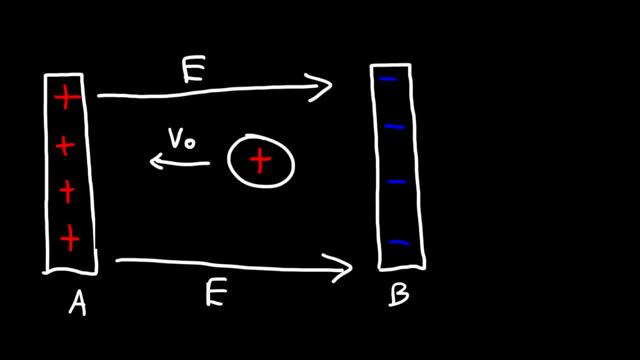 At this instant of time, as it moves initially to the left, the electric field still exerts a force that is parallel to itself. So the electric force acting on this charge is still directed towards the right. And it makes sense, because The charge 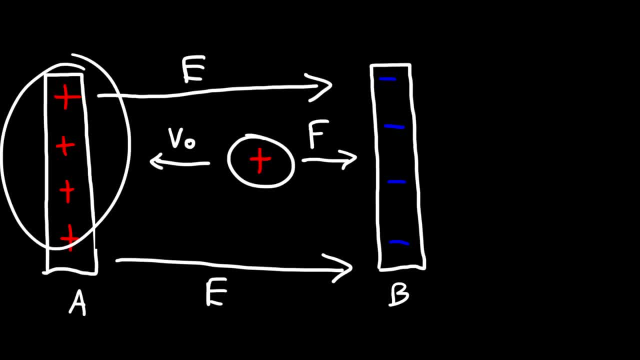 The positive charge is repelled by the positively charged plate, But it's attracted to the negatively charged plate, And so, even though it's moving to the left, due to its initial momentum it feels an electric force that is pulling it towards the right, towards the negatively charged plate. 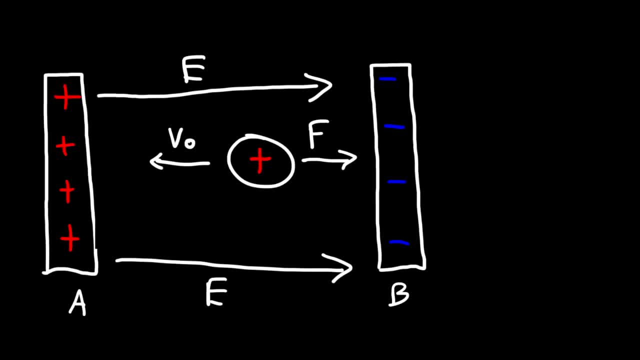 Because opposite charges attract each other, And so, right now, the charge has a displacement vector to the left, But the force Is towards the right, And so because the force and the displacement vector are anti-parallel or opposite. based on this equation, work equals force times displacement. the work done on this charge. 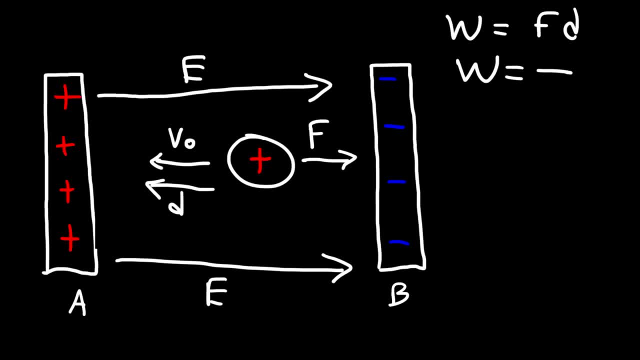 by the electric field is negative. So what does that mean? If the work done is negative, that means that the kinetic energy is decreasing. If you recall from the work-energy principle, Work is equal to Change in kinetic energy, And when the kinetic energy goes up, the potential energy goes down. 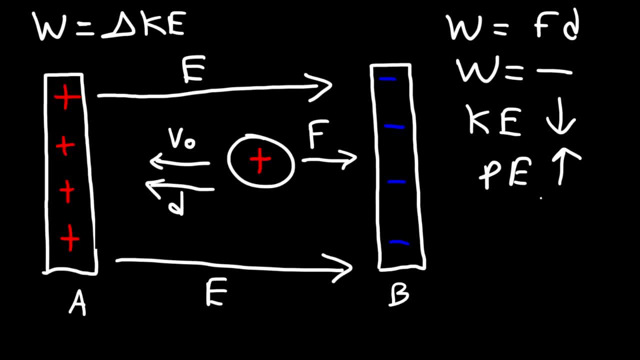 And if the kinetic energy goes down, the potential energy is going up. So the change in kinetic energy is equal to the negative change in potential energy. So in this case this charge is losing kinetic energy. It's slowing down. However, its potential energy is increasing. 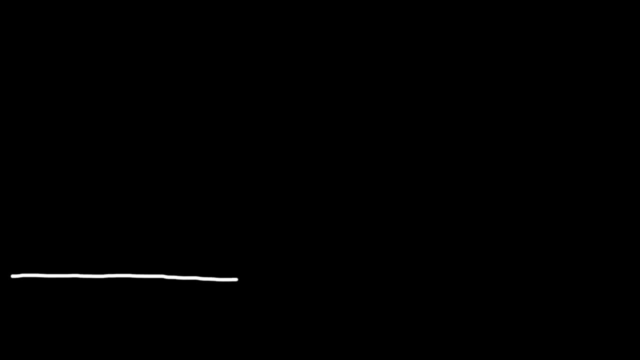 Now This situation is analogous to, Let's say, if we have a ball placed above the ground At this point above the ground, it has high potential energy And the ground has low potential energy, And so, as the ball falls from a position of high potential energy to low potential energy, 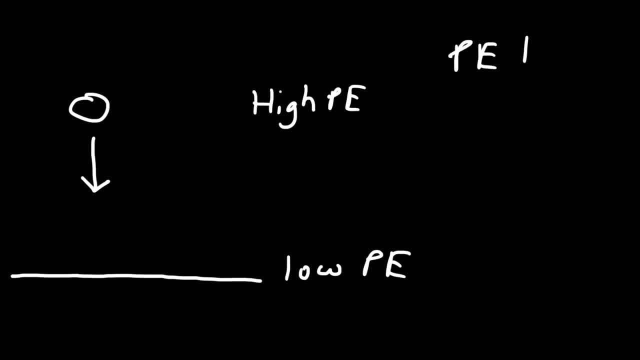 we could say that its potential energy is decreasing. So the energy is decreasing, And so the energy is decreasing. It's slowing down, but it's speeding up as it falls to the ground, and so the kinetic energy is increasing. Now this ball is falling down. 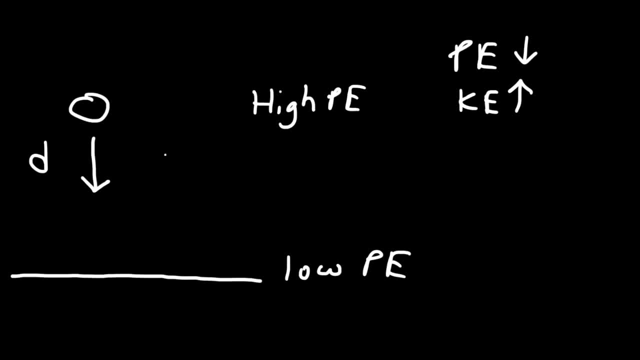 so its displacement vector is negative. It's going in the negative y direction. But the gravitational force acting on this ball is also in the negative y direction. So because the force and the displacement vector are in the same direction, the work done on this object is positive. 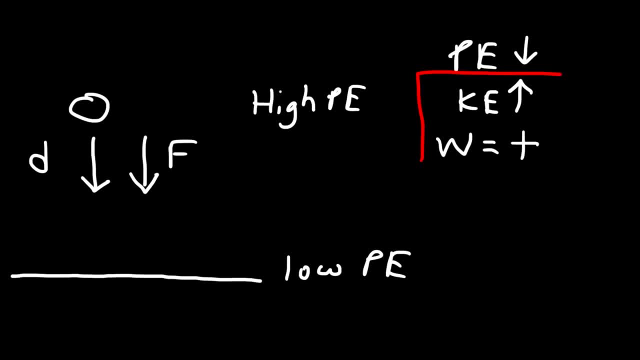 And any time the kinetic energy is increasing, the work done on that object is positive. So if the change in Ke is positive, the work done on that object will be positive. So this situation where the ball is falling towards the ground is analogous to this situation. 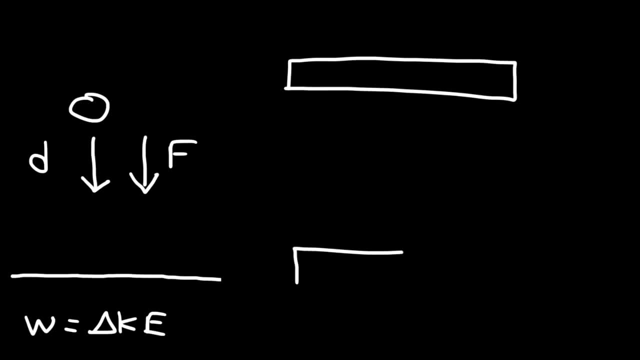 Let's say, if we have a positive place, we have a negative plate at the top and a negative plate at the bottom. A positive plate has more potential energy than a negative plate, So this would have high potential energy and this will have low potential energy. 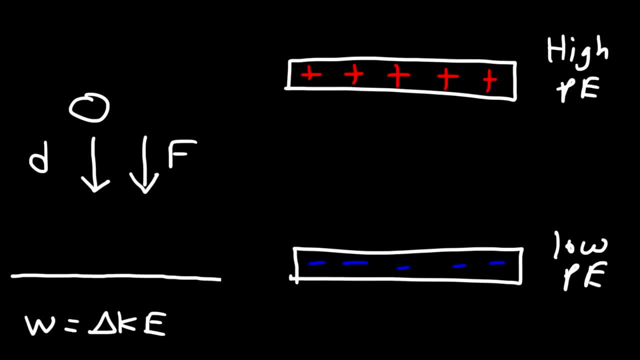 Now, in the case of the ball falling to the ground at the top, it has high gravitational potential energy. But when dealing with charges we need to say electric potential energy. Sometimes you'll see me write EPE for that. 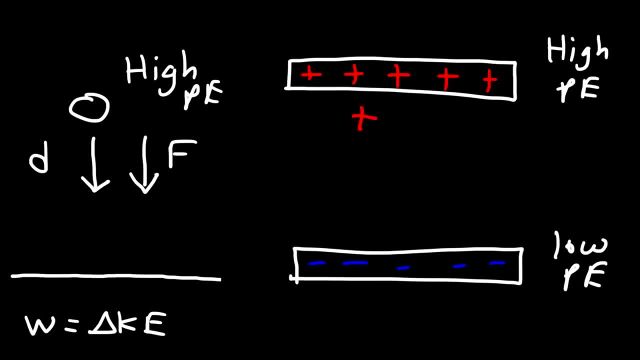 Now, as the positive charge, let's say, if we place it at the top, it's as we know, it's going to accelerate towards the negatively charged plate And so it's also moving in that direction and it feels an electric force pulling it in that direction. 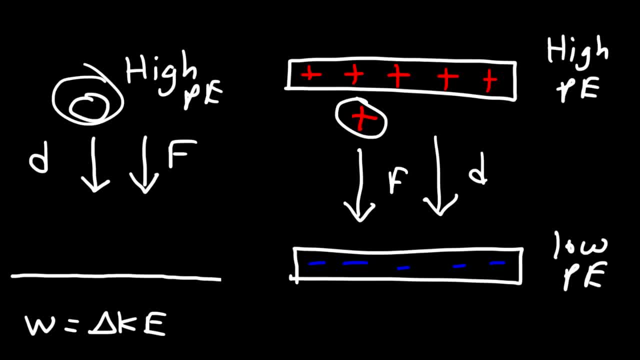 And so, just like the ball falling towards the ground, we know that the work is positive. That is, the work being done on the positive charge and on the ball, And the kinetic energy is increasing because it's speeding up And as it moves, from high potential energy. 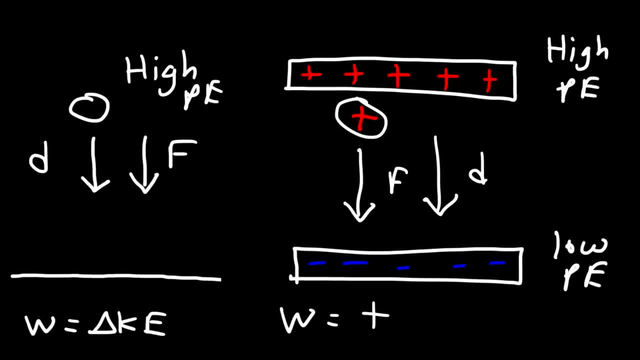 to low potential energy. the potential energy is decreasing. Now we talked about another scenario where a positive charge was given an initial velocity towards the positively charged plate, But it still feels a force that accelerates it towards the negatively charged plate, Because a positive charge will always feel a force. 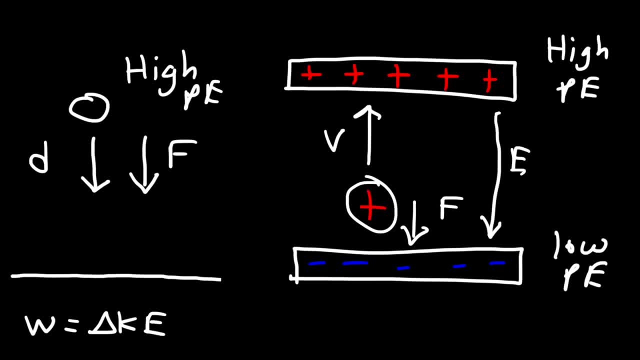 in the same direction as the electric field. For negative charges it's opposite to that. So in this case we said that because the force and displacement vectors are anti-parallel, the work done on this charge is negative And as it goes up, 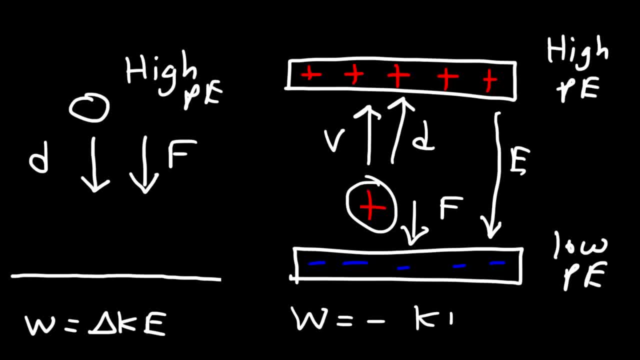 but the force is trying to bring it down. it's slowing down, So the kinetic energy is decreasing, but the potential energy is increasing because it's moving towards a position of high potential energy, That is, a position of high electric potential energy. Now the same is true for the ball, in this case. 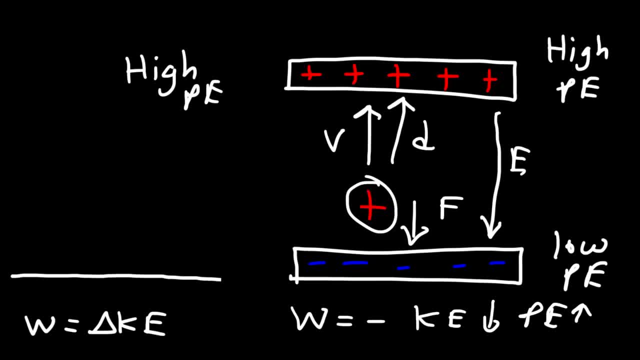 So imagine if you throw a ball upward in this direction. Actually, let me draw it here. So let's say the ball is going up, It has an initial upward velocity. Gravity is still acting on the force to bring it down. Now the ball, because it's moving up. 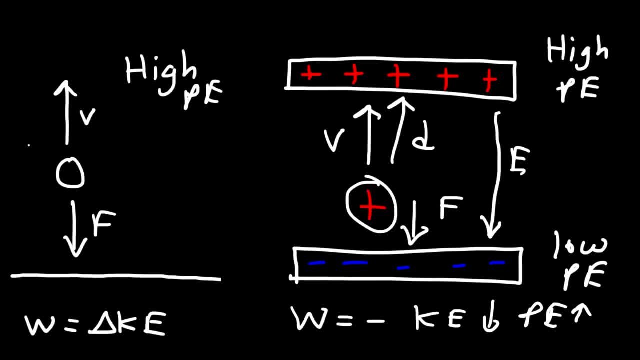 it has an upward displacement vector. So because these two are opposite to each other, the work done on this ball is negative. As the ball moves towards a high position, it's moving towards higher potential energy. So the ball is moving towards a higher potential energy. 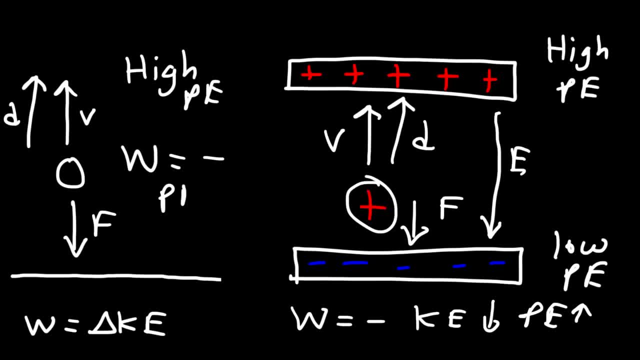 So the ball is moving towards a higher potential energy. So the ball is moving towards a higher potential energy. So the potential energy of the ball is increasing, But as it goes up it's slowing down and eventually it's going to reverse and go back to the ground. 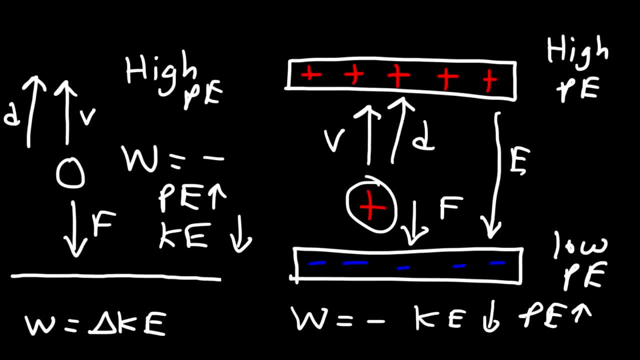 So, as it's going up, it's slowing down, Its kinetic energy is decreasing, And you can see the situation is the same here. And so by relating these two concepts, you can tell if a charge is going to, if positive work is being done on the charge. 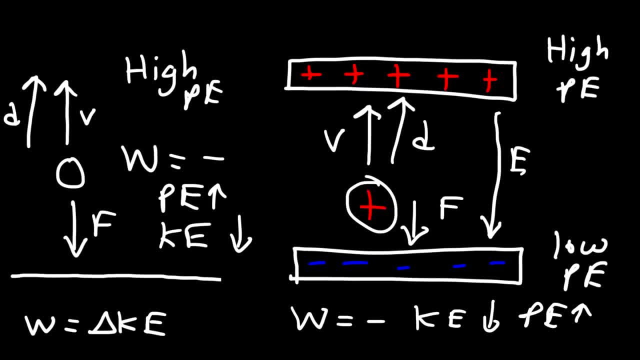 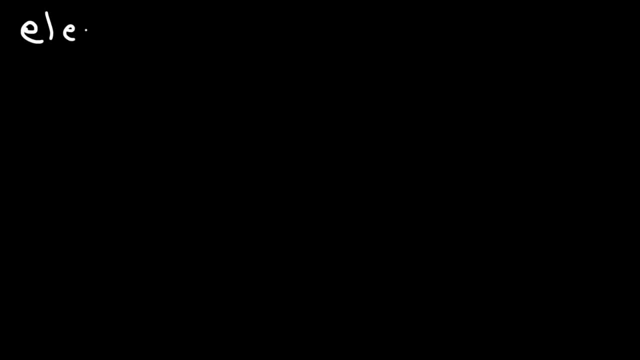 or if negative work is being done on it And if it's beaten, we're slowing down. Now we need to visit something called electric potential. electric potential- This is the next topic that you need to learn, after electric field っ. So what is meant by the term electric potential? 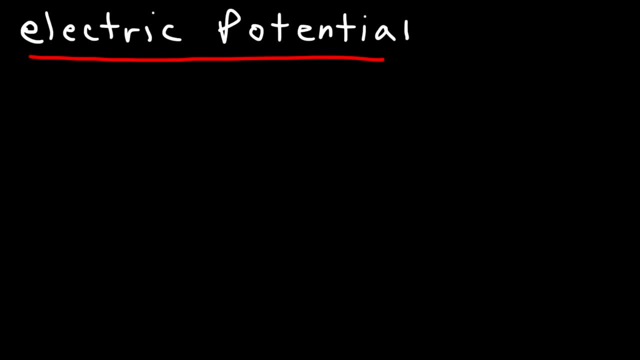 Electric potential represented by the symbol V. Electric potential represented by the symbol V is the ratio between the electric potential, energy and electric field. if you tried to find what those are, of the charge and the magnitude of the charge, The unit for electric potential V. 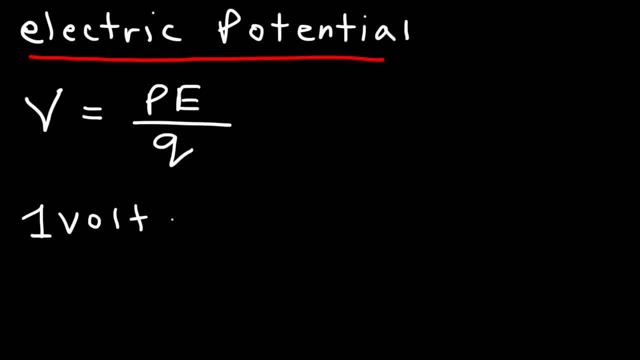 is the volt, And one volt is equal to one joule of potential energy. that is, electric potential energy per one coulomb of charge, And a good way to understand the concept of electric potential is using those two plates again Now it's important to understand that the difference in electric 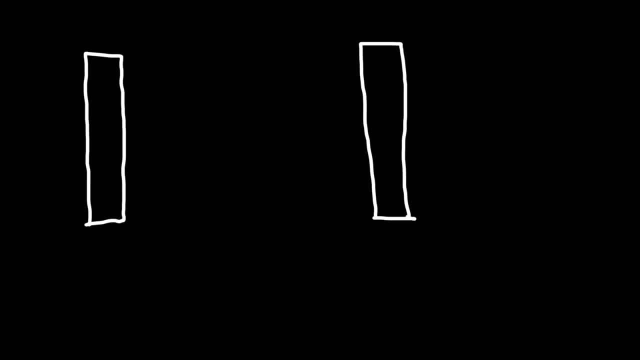 potential is really what can be measured, and so that's the important stuff. Electric potential itself is an arbitrary number. It's only useful if you compare it to the electric potential at another position. So let's say that the electric potential at the negatively charged plate- we're going to say it's 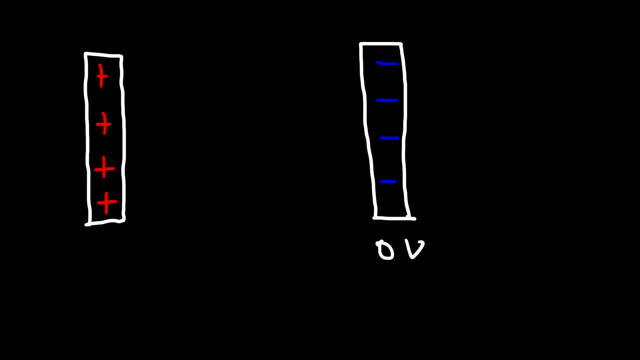 zero volts And the electric potential at the positively charged plate. let's say it's 100 volts. Actually, let's say it's 5 volts. Now let's say if we have a positive charge at position A, Let me move it close to this. 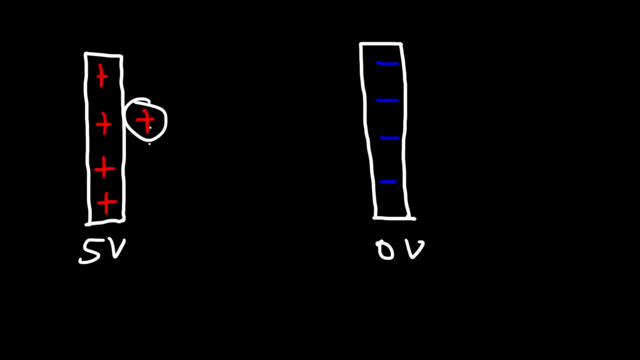 plate. So let's say it starts directly on the positively charged plate, which we'll call position A, And it accelerates towards the negatively charged plate. And let's say it's a one coulomb charge. So this one coulomb charge is moving. 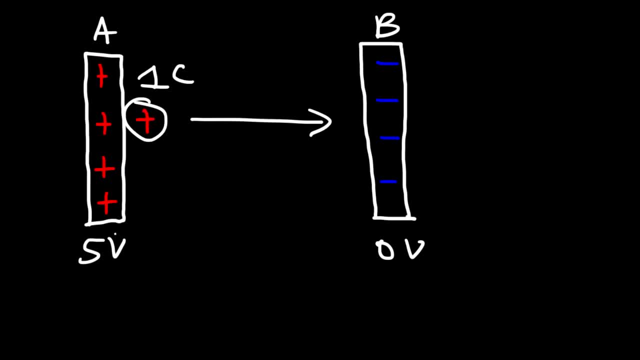 through a potential difference of 5 volts, from 5 to 0. And we know that it's going to gain kinetic energy During this process and it's going to lose potential energy. So in this case now keep in mind one volt represents one joule per one coulomb of charge. So when 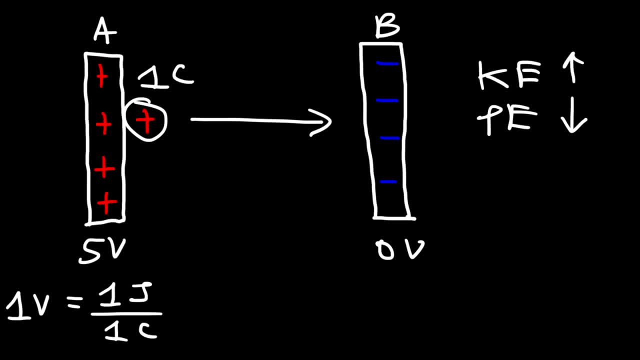 a one coulomb charge moves through a potential difference of 5 volts. 5 joules of work is being done on that charge. Now, whether the work be positive or negative, it depends on the situation. Is it moving from A to B or B to A? Now we know that, as 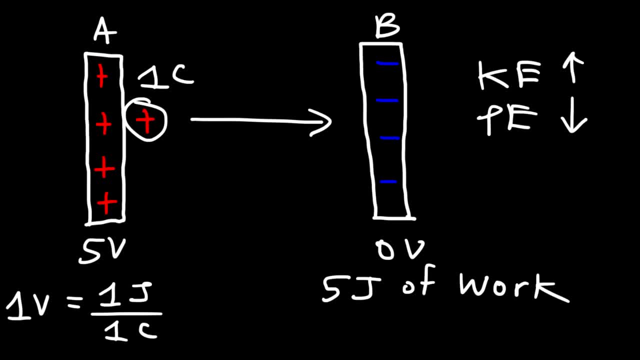 it moves from A to B, the kinetic energy is increasing. So therefore the electric field is doing 5 joules, that is, positive 5 joules of work on this one coulomb charge, And so we could say that the charge loses 5 joules of potential. 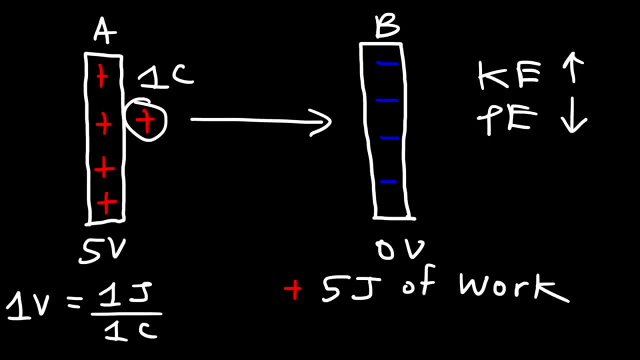 energy during this process, Or we could say that it gains 5 joules of kinetic energy. Now let's compare it to another charge, but this time we're going to say that this charge has 2 coulombs of charge and it's moving from A to B. In this case we could say that 10 joules of work. 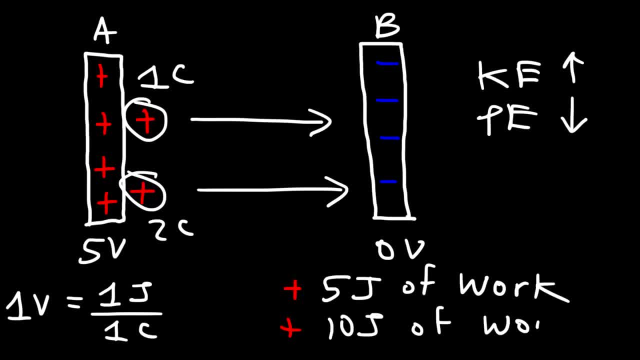 will be performed on this 2 coulomb charge as it moves from A to B, And so we could also say that it's losing 10 joules of potential energy or gaining 3 joules of kinetic energy, And so we could say that it's losing 10 joules of potential energy or gaining. 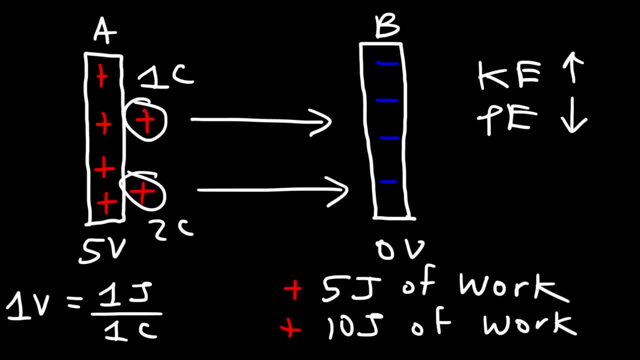 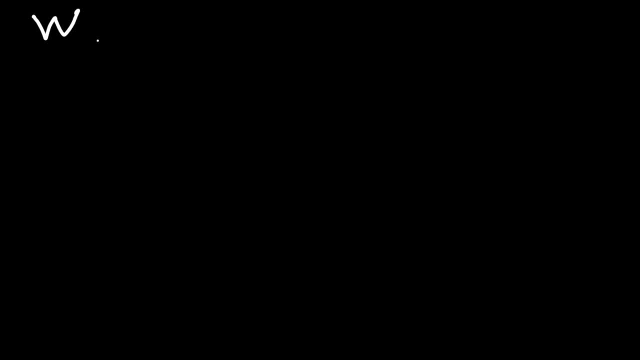 10 joules of kinetic energy. Now this leads us to an important equation. So the work done from moving a charge, let's say from B to A, is equal to negative Q times the electric potential difference between points A and B. So you could say it's equal to negative Q times VA minus VB. 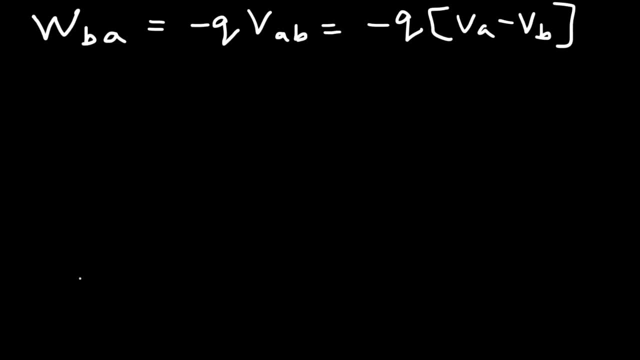 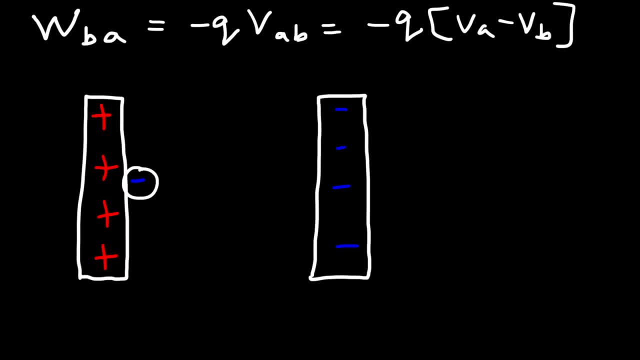 It's repelled by the negatively charged plate. But let's say we use an external force and force it in this direction. So this is not the force generated by the electric field. We're using an external force to move it, let's say, from A to B. 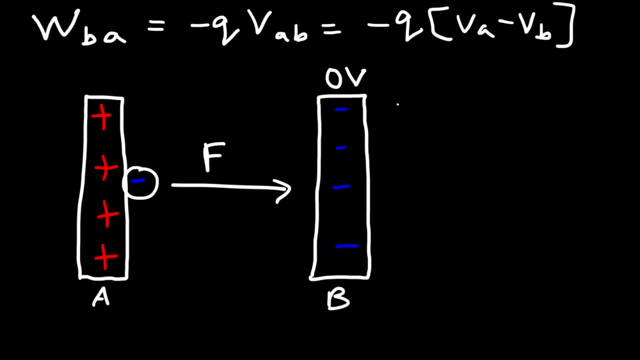 Now let's say the potential at this plate is zero and at this plate is 50. now let's say this is just a negative charge, not necessarily an electron, but there's many electrons, and so let's say the total charge of that object is 20 microcoulombs. 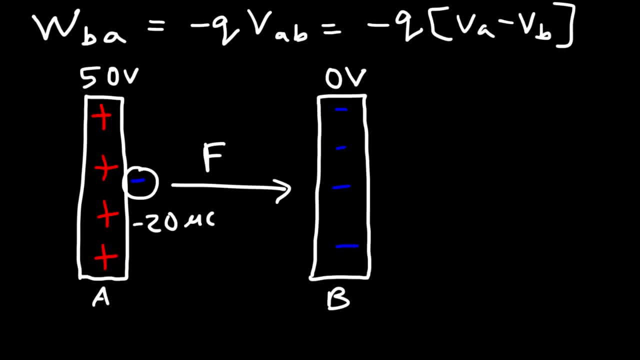 but it's going to be negative. though how much work is done by moving a charge from A to B, and is the work positive or negative? so right now, the displacement of the negative charge is towards the right. the electric field is also towards the right, but a negative charge will feel an electric force. 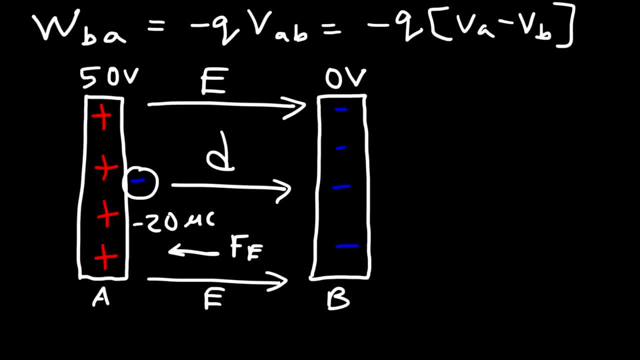 that will accelerate it in the opposite direction of the electric field. so even though we're using an external force to move it from A to B, the negative charge still feels an electric force that will attract it or pull it towards the positive plane. so let's say that we have a negative charge. 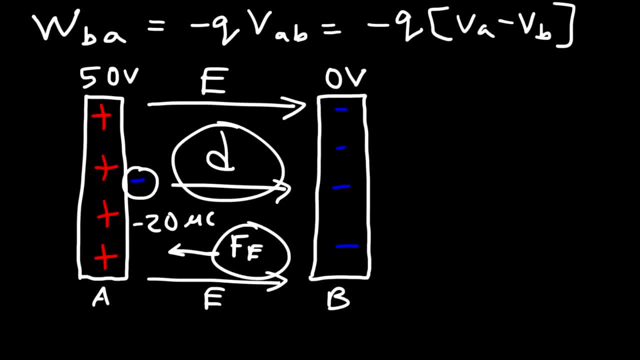 now, because the electric force and the displacement vector are anti-parallel, the work done by the electric force is negative. now let's see if we can quantify this answer. now we're going from A to B and not B to A, so this equation is going to change. 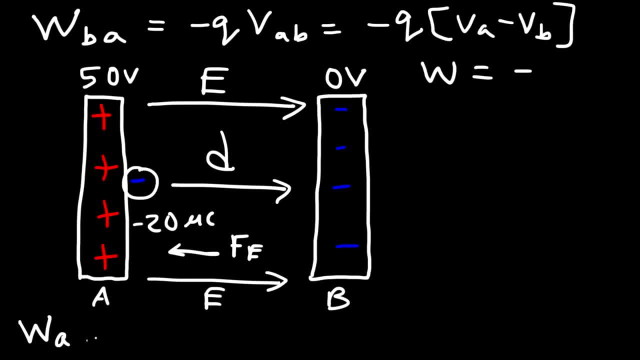 so we're going to say the work done on the charge going from A to B is equal to- and I'm going to focus on the electric force and I'm going to focus on this portion of the equation- negative Q times the electric potential difference between point B and point A. 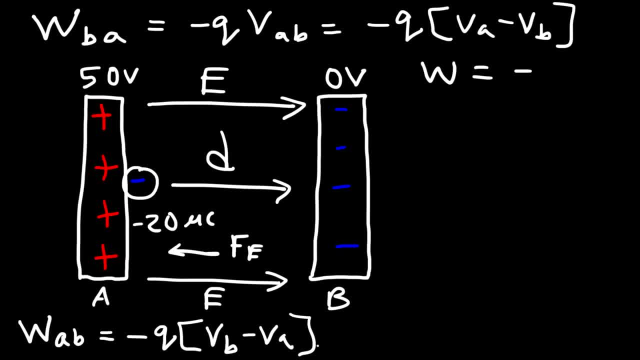 so VA is the electric potential at point A, VB is the electric potential at point B. but it's the difference in electric potential that really matters. and you know what? let's change the charge. instead of using micro, let's use a nice whole number. let's say: 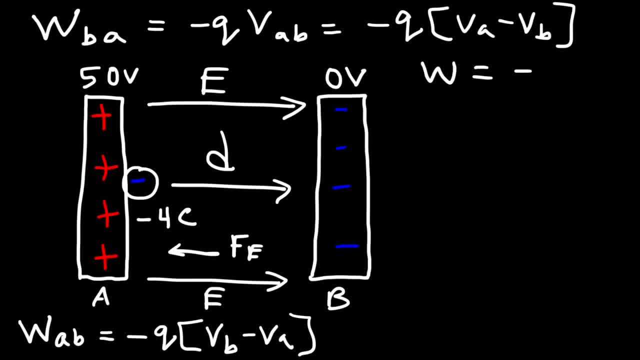 negative Q times the electric potential negative 4 coulombs. now, if you recall, whenever a charge moves to, let's say, a potential difference of 1 volt, a 1 coulomb charge will have 1 joule of work done on it. it could be positive or negative. 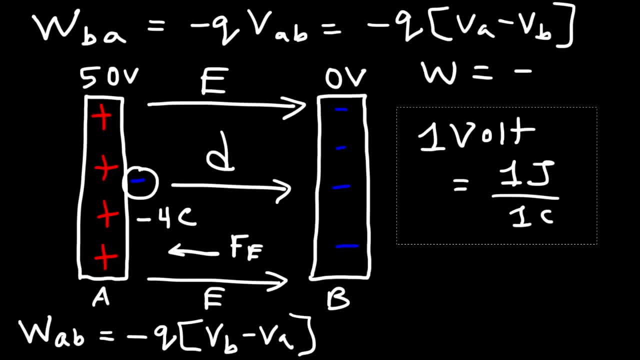 but it's going to be 1 joule of work. in this case we have a 4 microcoulomb charge moving through a potential difference, so let me write delta V of 50 volts, and so in this case it should be about 200. 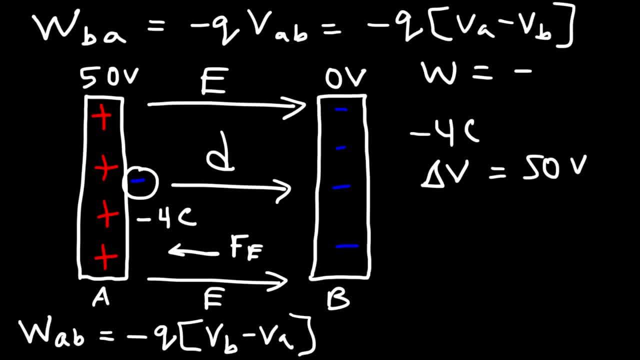 because a potential difference of 50 volts means that the charge can gain or lose 50 joules of energy per 1 coulomb of charge. so it can gain 200 joules of energy or lose 200 joules of energy per 4 coulombs of charge. 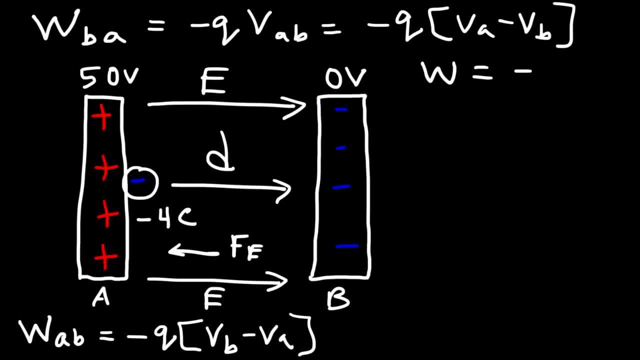 so, using this formula, we have negative Q. now Q is negative 4 coulombs because we're dealing with a negatively charged particle or object and VB, the potential at point B is it's 0, the potential at point A is 50, so we have 2 negative signs. 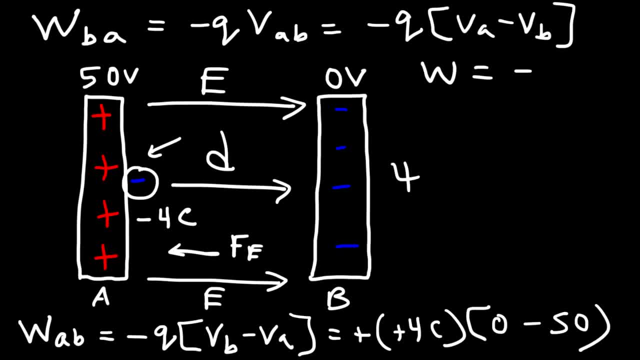 a negative times. a negative is a positive and 0 minus 50 is negative 50. so overall, this is going to be, this is going to be negative. so it's negative. 200 joules of work being done on this negative charge and so, just as we predicted, 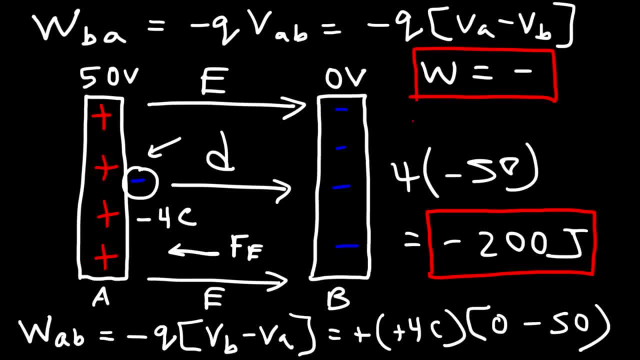 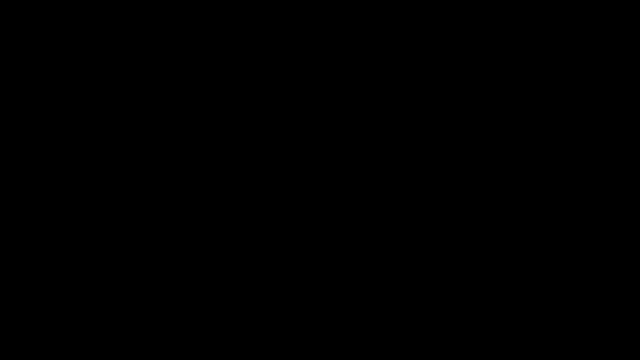 the work was going to be negative when the negative charge moves from position A to B. so hopefully this section gave you a good understanding of the concept of electric potential, energy and electric potential. so make sure you understand the difference between electric potential and potential. so I'm going to show you. 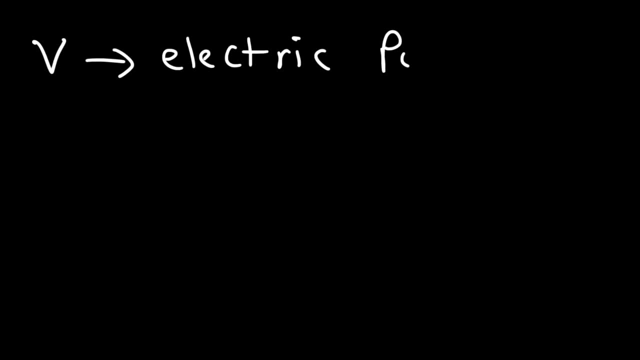 the electric potential in the answer. V represents electric potential without the word energy in it, just potential, and the unit for electric potential is the volt. so when you think of a 9 volt battery, what this tells you is that it can do 9 joules of work. 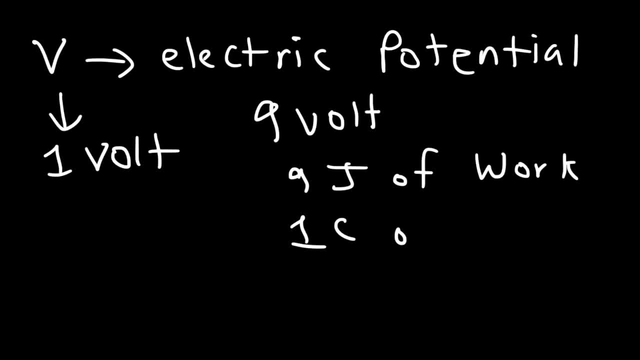 when it passes one coulomb of charge through a circuit. And so it helps you to understand the concept of voltage. Voltage is really the difference in electric potential. It's the change in the electric potential, So it's like VA minus VB or VB minus VA. 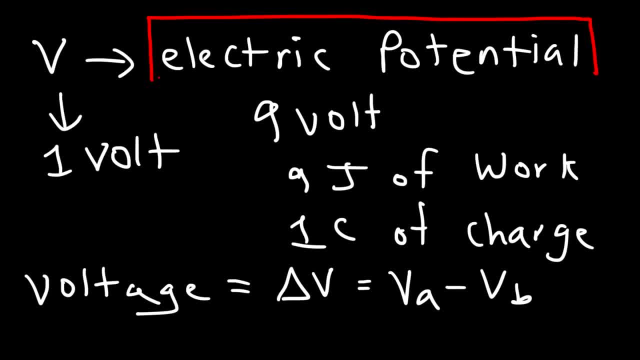 So electric potential is simply an arbitrary number. It's simply V, But delta V. that is a voltage which is more commonly used in everyday applications. So make sure you understand the difference between electric potential and voltage, And also electric potential, energy, which is PE.